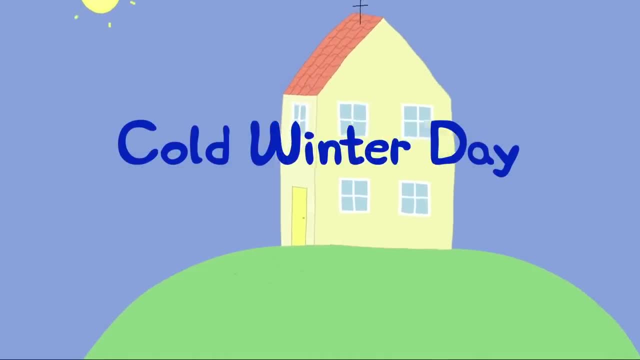 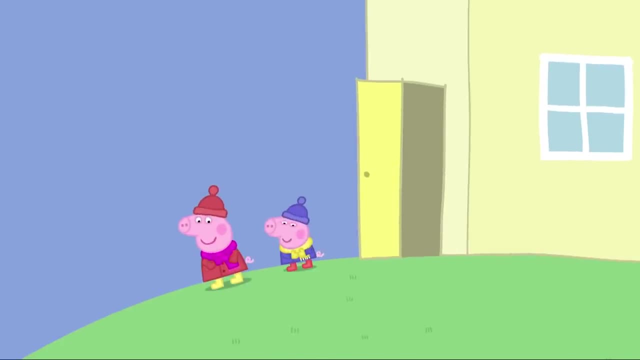 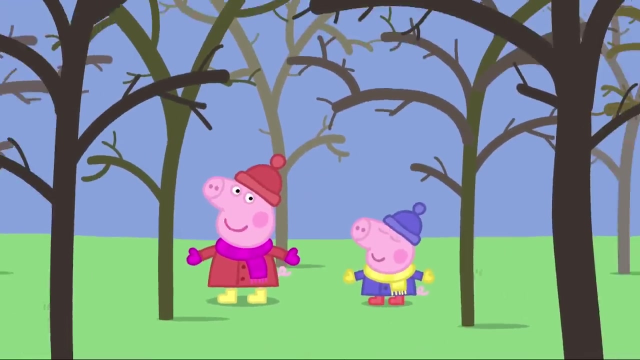 Cold winter day. It is very cold today. Peppa and George are wearing their hats, scarves, coats, mittens and boots. Look, George, The trees haven't got leaves. In the wintertime, the trees lose their leaves. 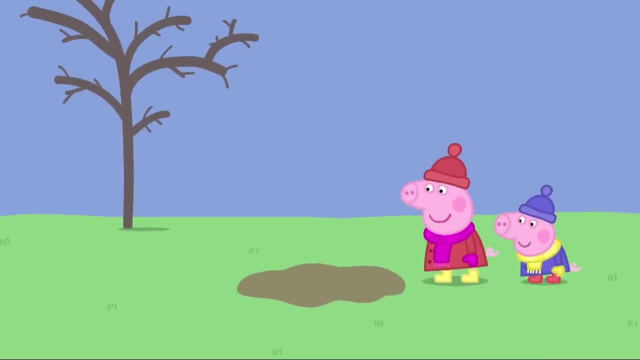 Peppa and George have found a muddy puddle. Peppa and George love jumping up and down in muddy puddles, Me first. It is so cold the puddle has turned to ice. It is very slippery. It's not funny. 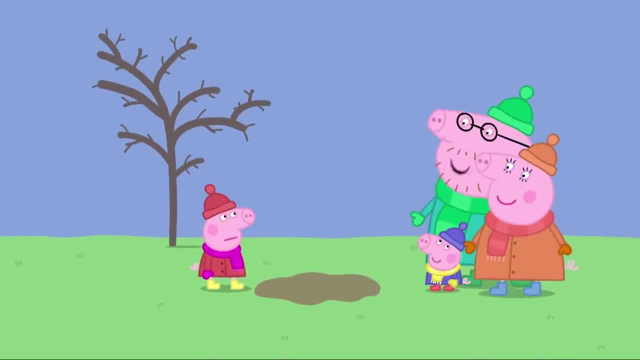 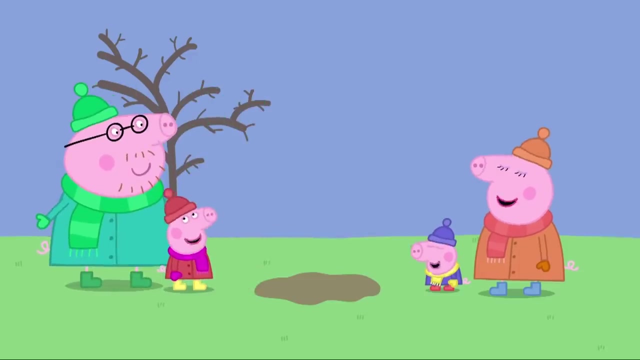 Here are Mummy Pig and Daddy Pig. Oh good, A muddy puddle. Daddy Pig loves jumping in muddy puddles. Stop, Daddy. That was close. Lucky I've got such a good sense of balance. Daddy, the puddles are icy today. 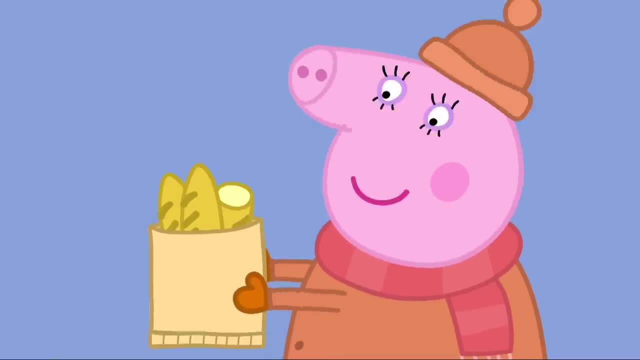 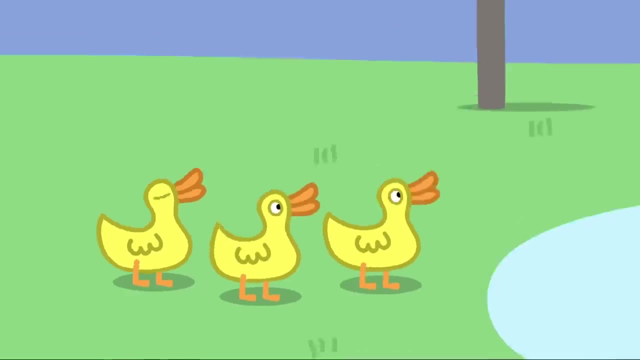 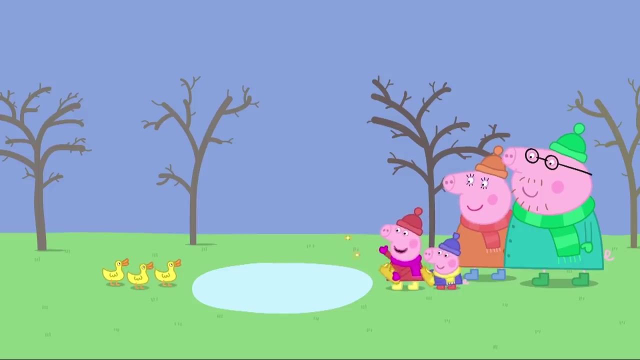 We can't jump in them, Never mind, Let's feed some bread to the ducks. Hooray, Peppa and George love feeding the ducks. Hello, ducks, We've got some bread for you. The ducks like bread Oh. 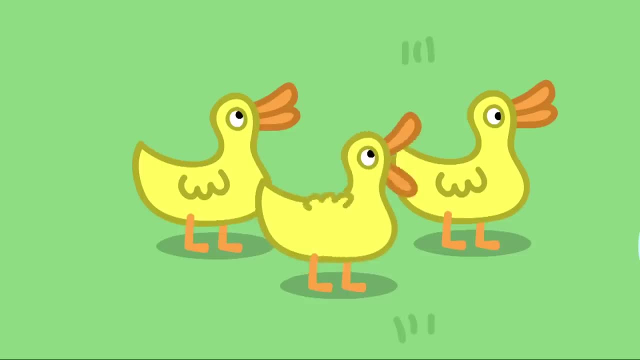 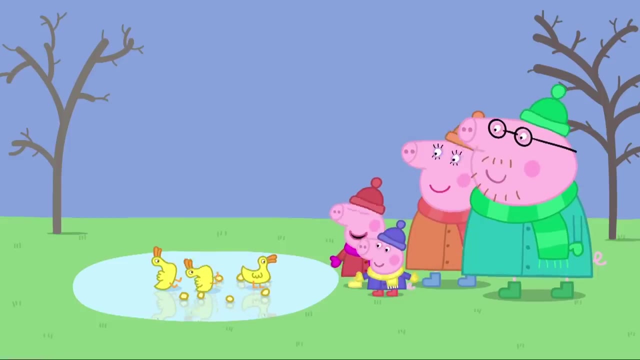 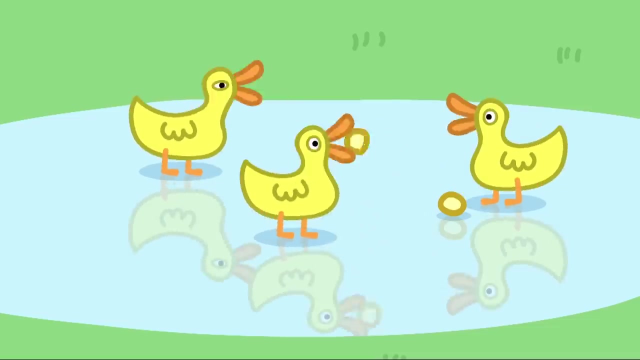 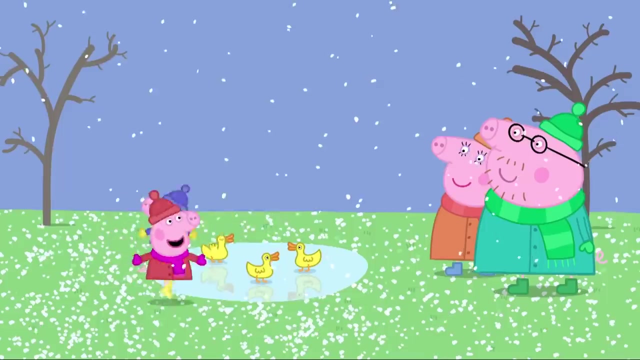 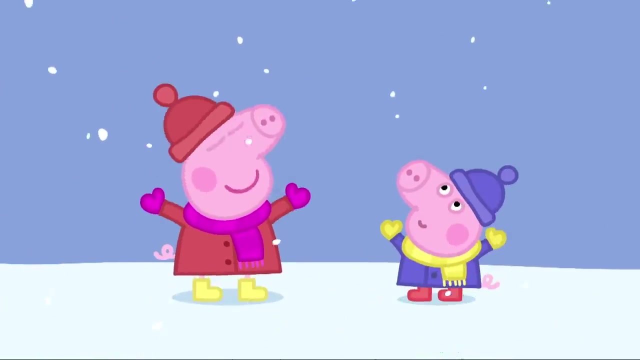 It is so cold the pond has frozen to ice. The ice is very slippery. Sorry for laughing, Mrs Duck, but it did look quite funny. It is starting to snow Snow. Peppa and George love snow. George, let's catch snowflakes. 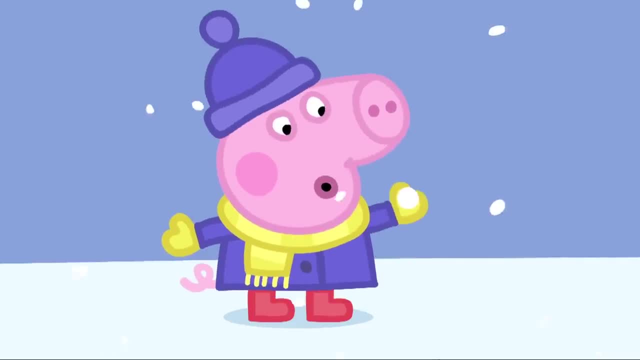 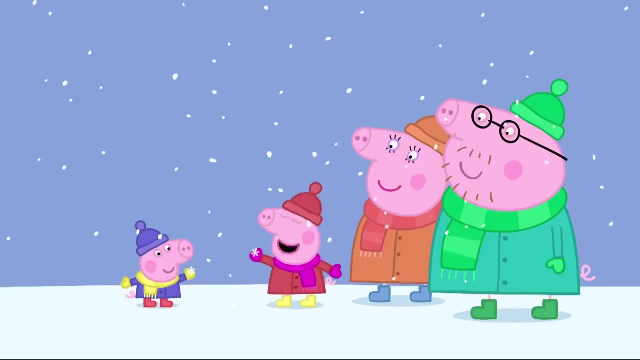 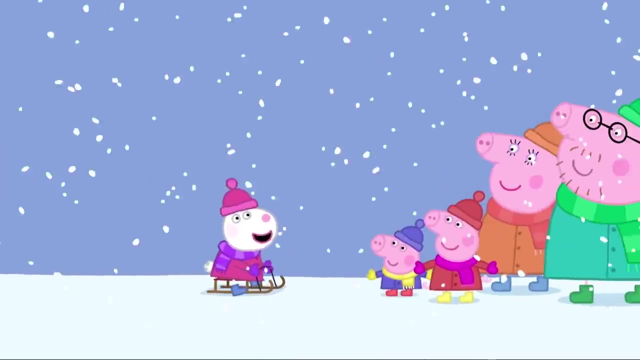 Peppa and George are catching snowflakes. George has caught a snowflake. Peppa has caught a snowflake. Ooh, Here is Suzy Sheep on her toboggan. Whee, Hello, Peppa. Wow. 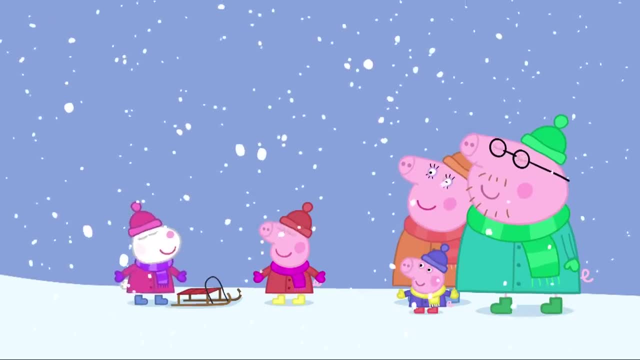 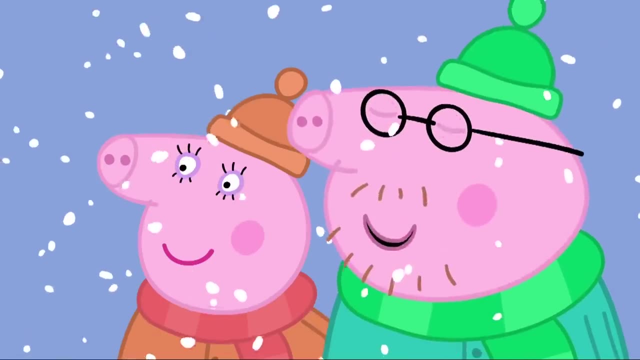 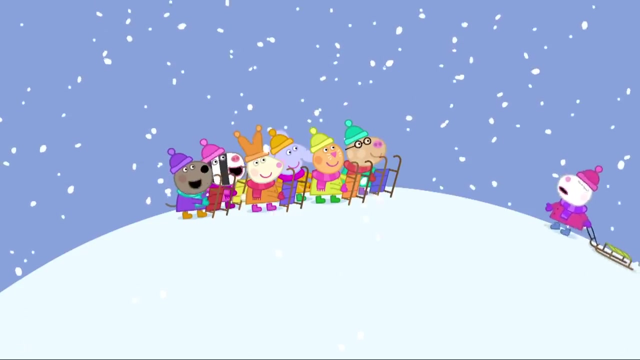 Suzy, that looks fun. We're all toboggans. We're all tobogganing on the big hill. There's lots of snow there. Shall we climb up the big hill and watch the tobogganing? Yes, please. Peppa's friends are tobogganing on the big hill. 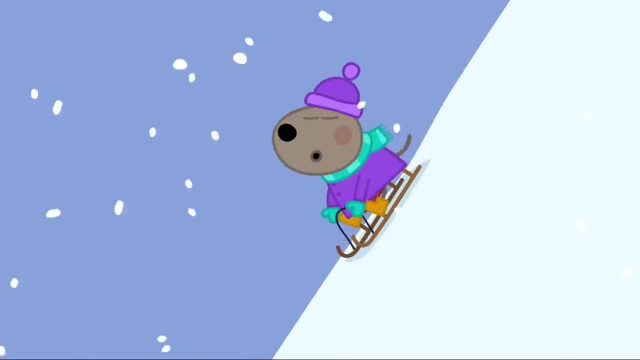 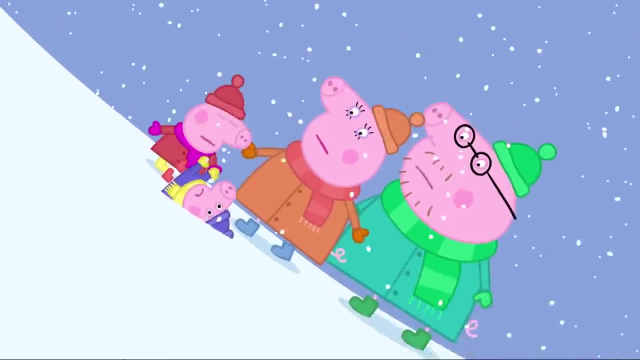 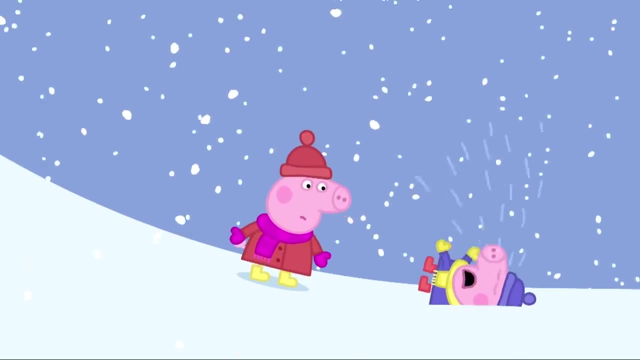 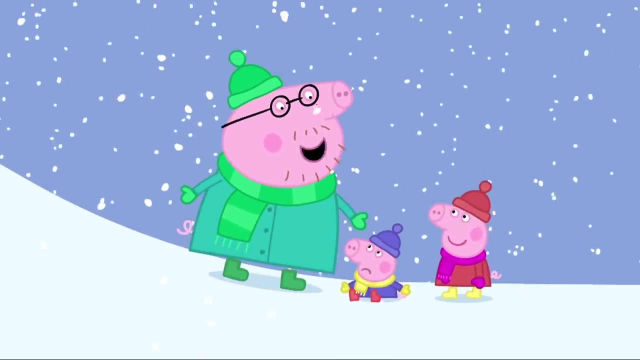 Whee, Yahoo. Oh, dear George has slipped on the hill. You look funny, George. George does not think it is funny. It's quite easy to slip on the hill. Maybe I should carry George Daddy, can you carry me too? 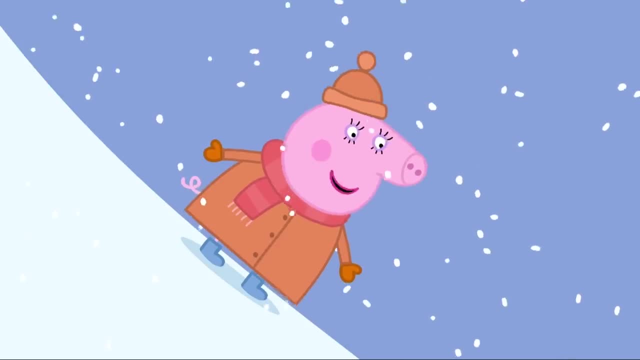 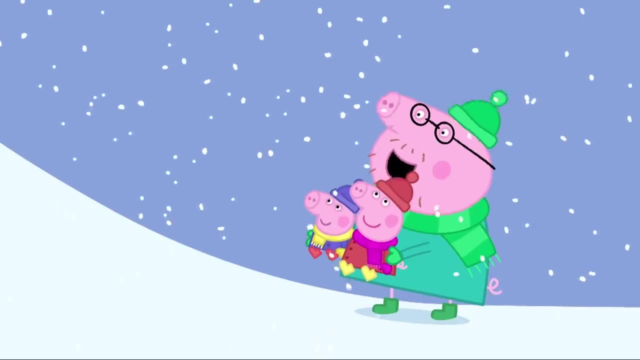 Ho ho. All right, Peppa, Just be careful you don't slip over Daddy Pig. Ho ho, Don't worry, Mummy Pig, Remember, I've got an excellent sense of balance. I'm going to have fun. 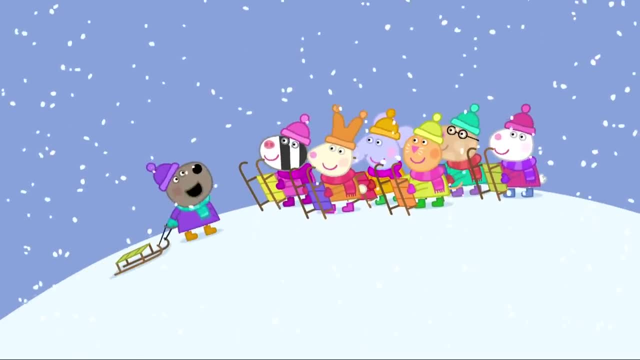 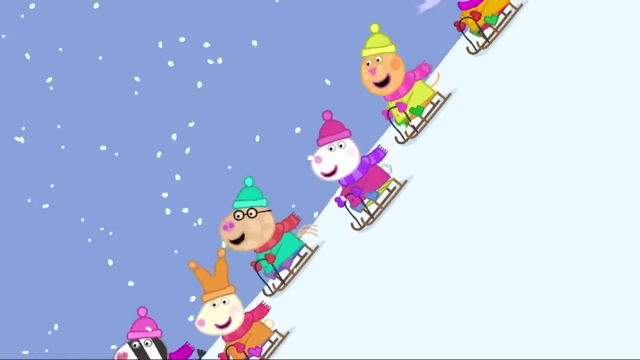 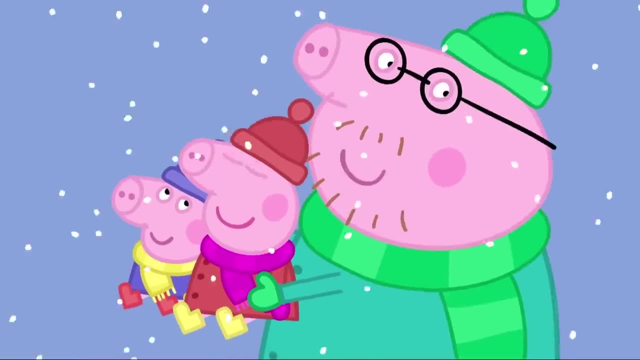 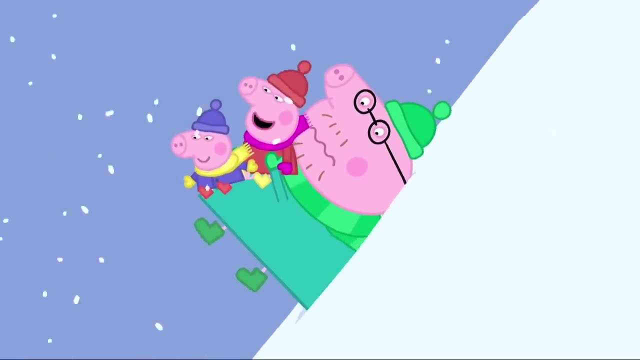 Do be careful you don't slip Daddy Pig. Ho ho ho, I'm not going to slip. Whoa, Whoa, Ha ha ha. Daddy is like a big toboggan, Ha ha ha. 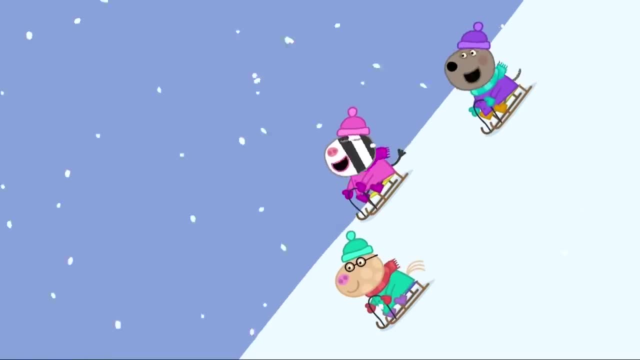 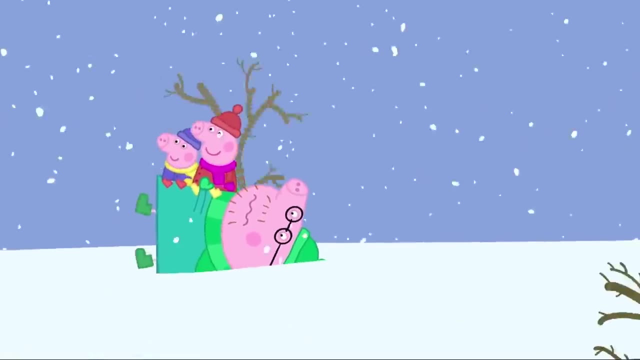 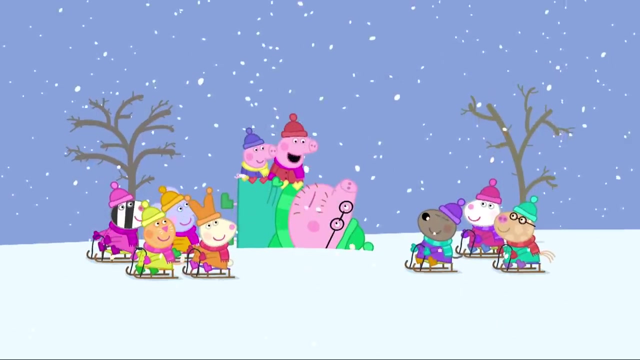 Whoa Whee, We're going to win the race. Hooray, Peppa and George are the winners. Well done, Peppa. My daddy makes a very good toboggan. It's not funny. It is a bit funny, Daddy Pig. 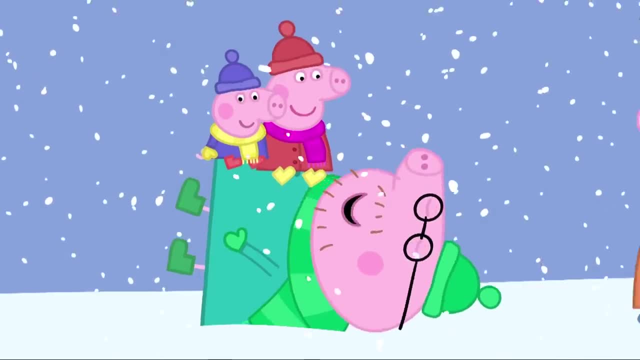 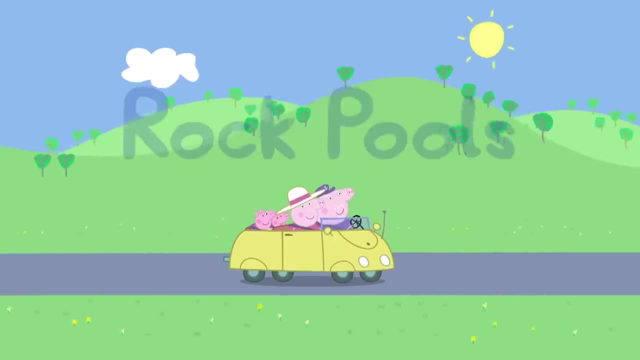 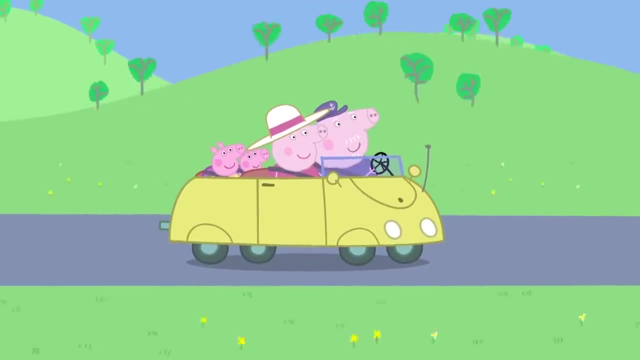 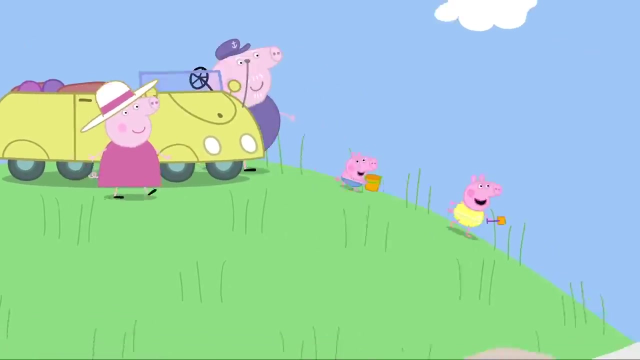 Hmm, I suppose it is quite funny. Ha ha, ha, ha ha. Rock pools. Peppa and George are going to the seaside with Granny and Grandpa Pig. Ha ha, ha, ha ha. Peppa and George love the seaside. 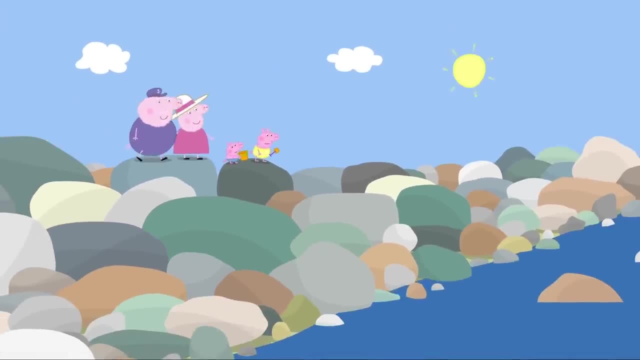 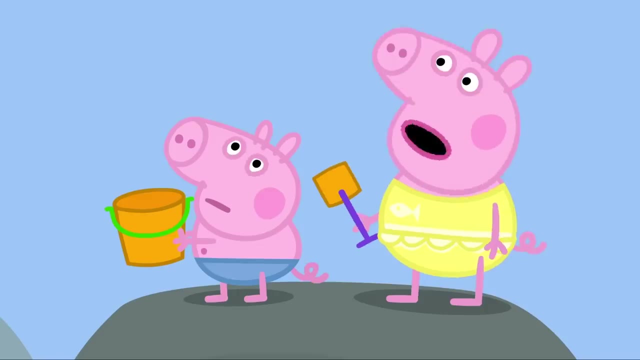 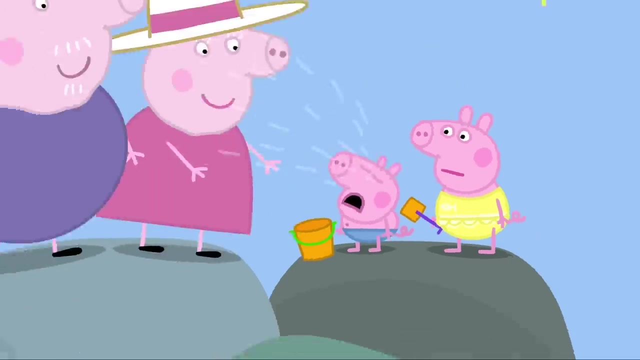 Oh, where's the sand gone? There isn't any sand. There isn't any sand on this beach, Peppa. No sand. But we wanted to make sandcastles. Peppa and George love making sandcastles. Now, now, George, don't be upset. 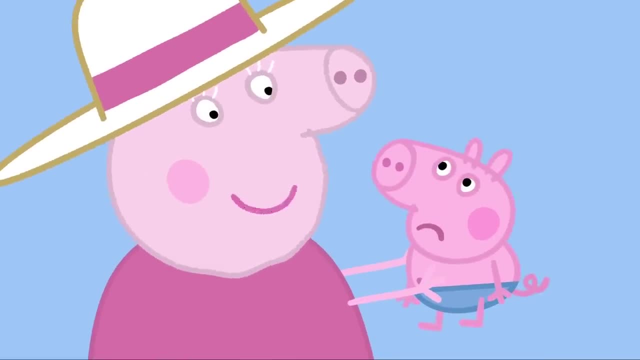 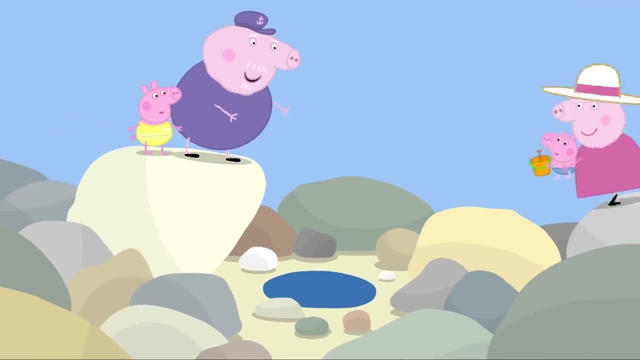 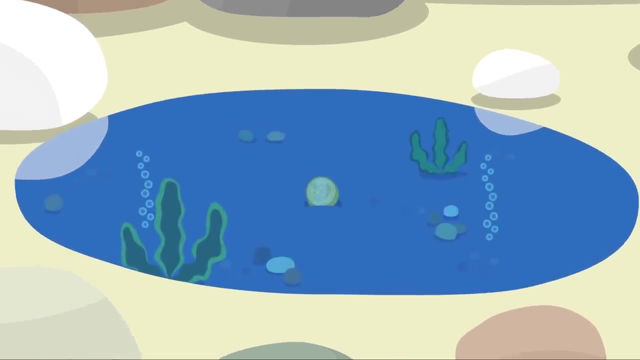 There are lots of exciting things to do on this rocky beach. Like what? When the sea goes out, it leaves little pools of water in amongst the rocks. They're called rock pools, And in every rock rock pool there's something special that the sea has left behind. 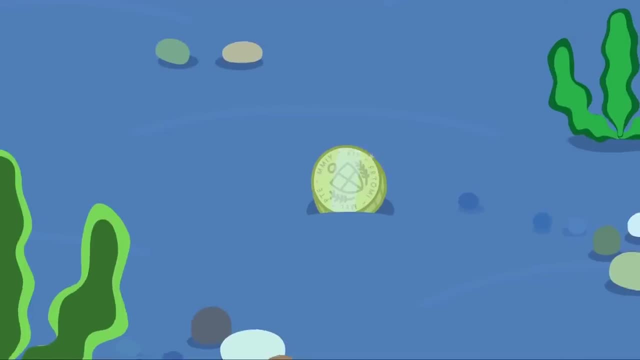 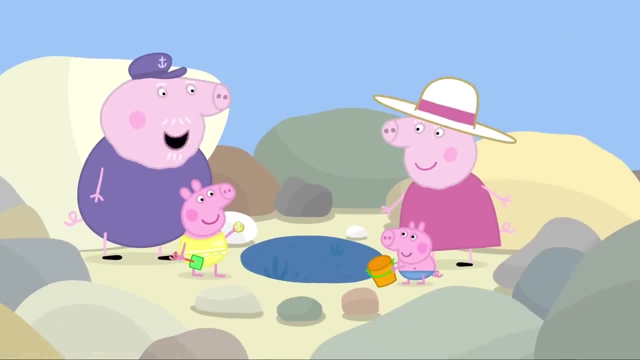 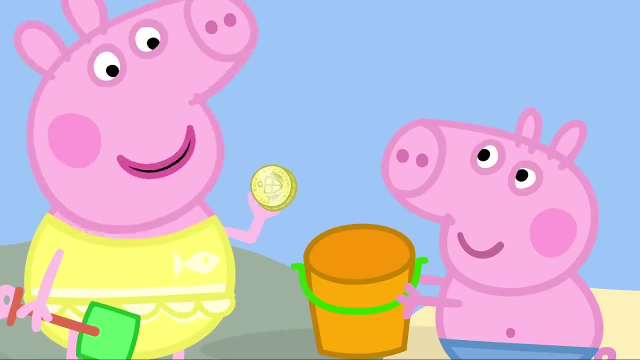 Ooh, I can see something glittering. It's a coin. Wow, Maybe it's a pirate's treasure. Ooh, Let's make a collection of all the things we find. Yes, We'll put them in George's bucket. 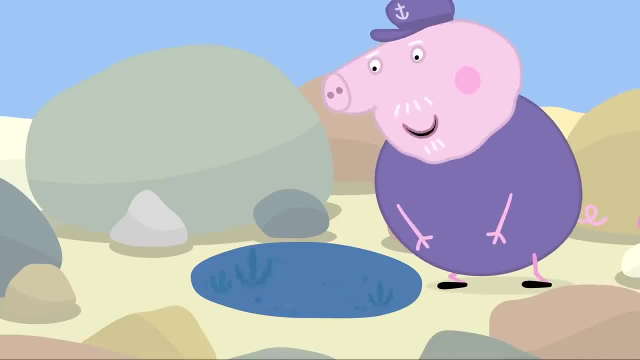 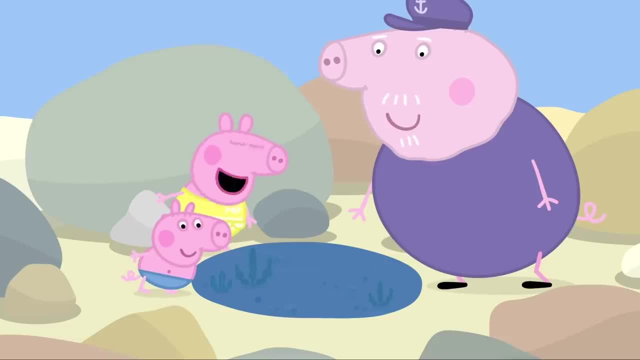 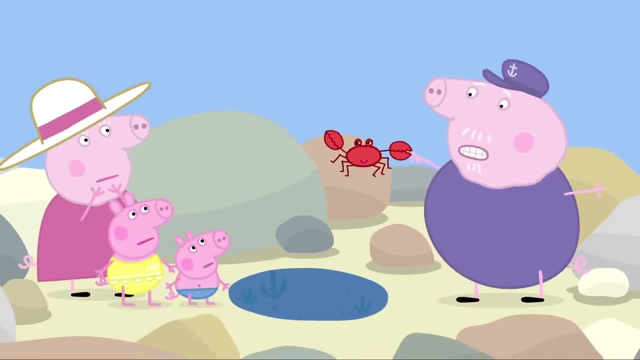 There's nothing special in this one. Ho, ho, ho, ho. There's always something, Peppa, Look closer. Ooh, There is something. Yes, It's a crab. Aaaahhh, The crab is pinching Grandpa Pig's finger. 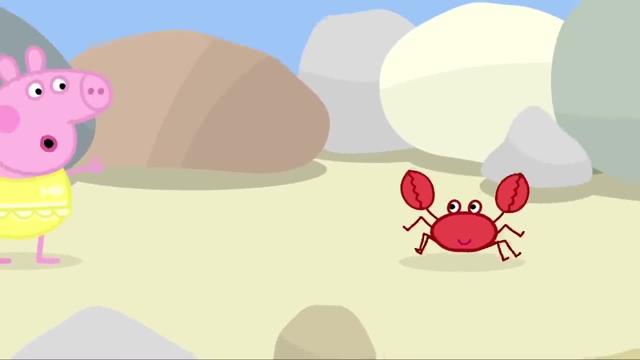 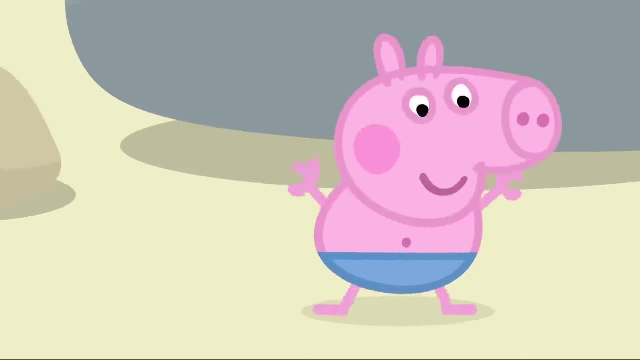 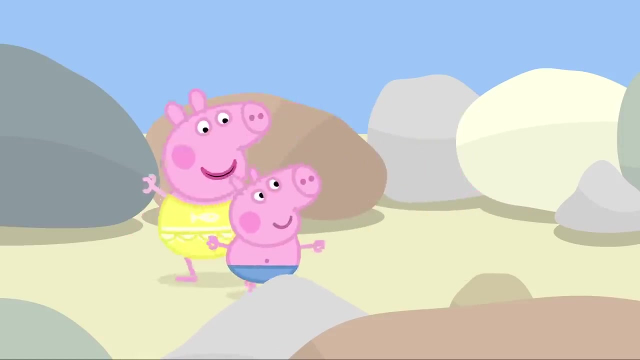 Ooh Ouch, Naughty Mr Crab. Mr Crab is walking sideways, George is pretending to be a crab, Peppa wants to be a crab too. We're naughty crabs. Pinch, pinch, pinch, Pinch, pinch, pinch. 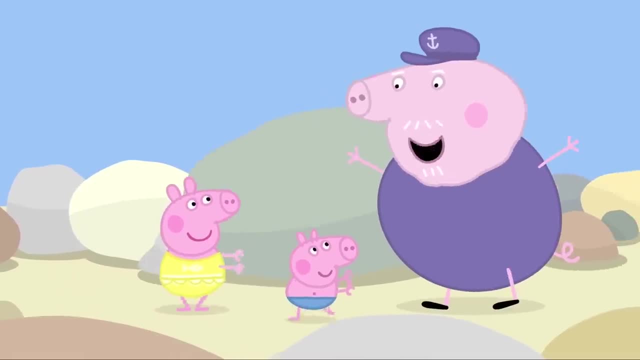 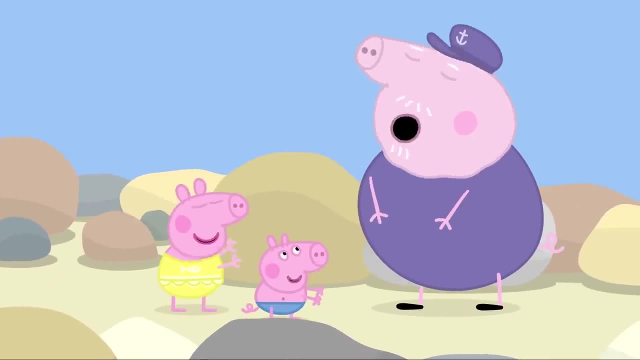 Help. There are two naughty crabs trying to pinch me. Pinch, pinch, pinch. We're naughty crabs, Pinch, pinch, pinch. Oh, Shoo, shoo, shoo. you naughty crabs Go back to your little rock pools. 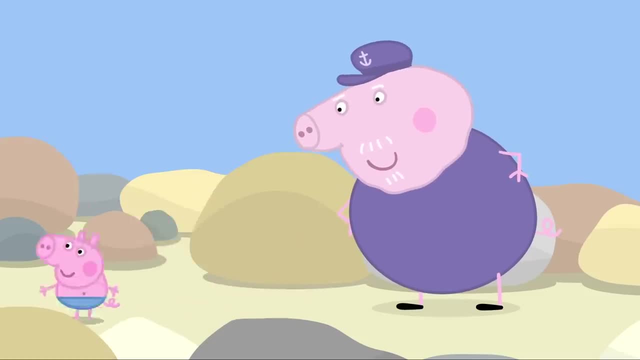 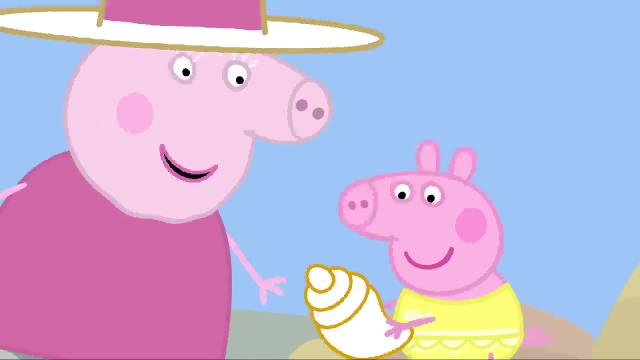 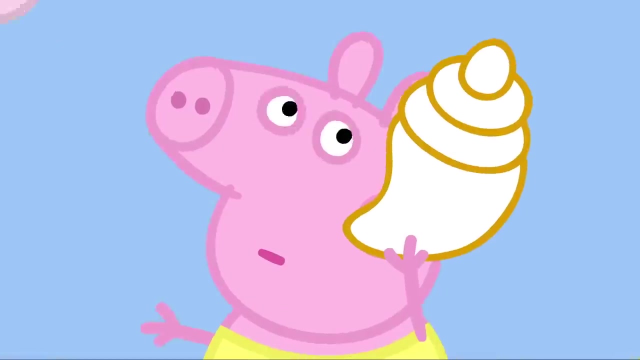 Yes, Let's look in more rock pools. What can you see? A seashell. Can you hear the sea in it? What do you mean? If you put a shell to your ear, you can hear the sea. Wow, I can hear the sea. 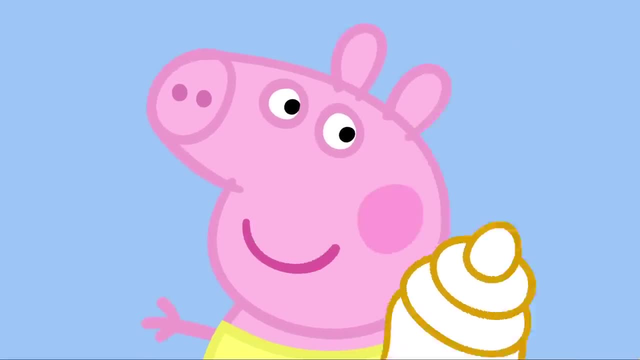 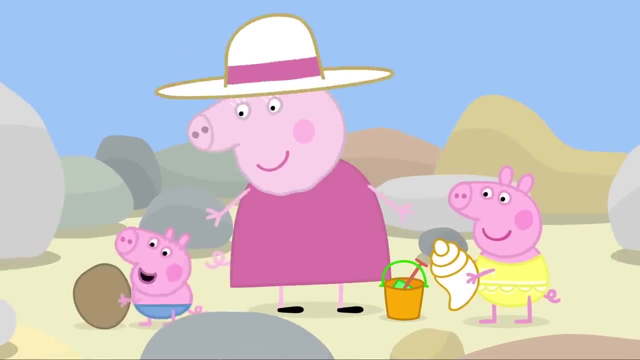 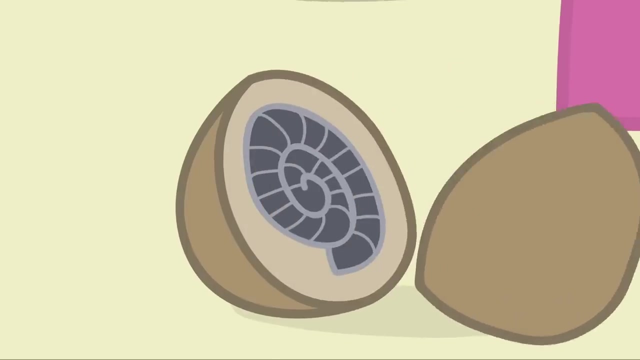 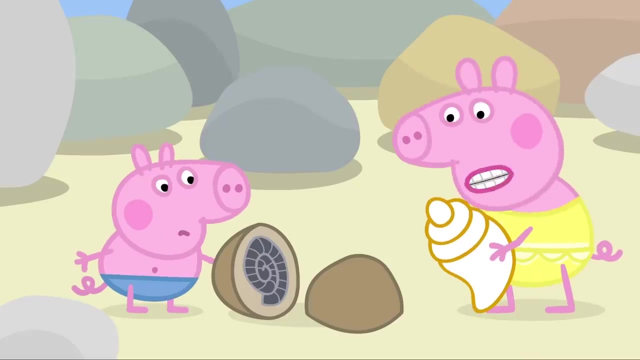 I love my seashell. George, can you find a seashell too? Shell, That's not a shell. Oh, Peppa's right, That's not a shell. George has found a fossil. What's a fossil? 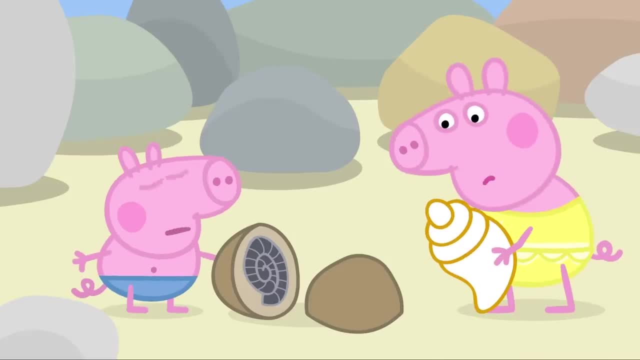 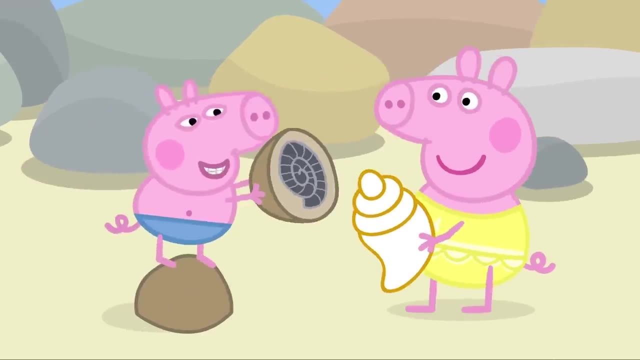 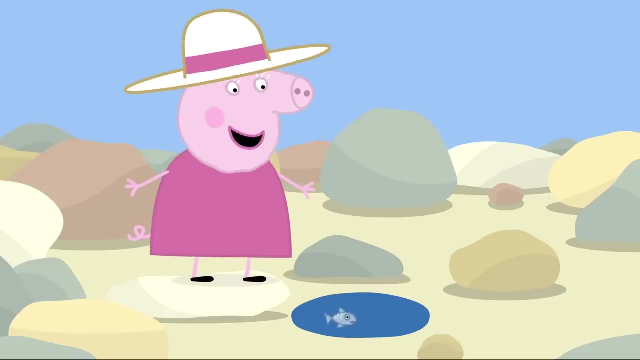 A fossil is the remains of an animal that lived long ago, When there were dinosaurs, Dinosaur Whoa Hee. Rock pools are such fun. Yes, They're fun for us, But not for this little fish, A fish. 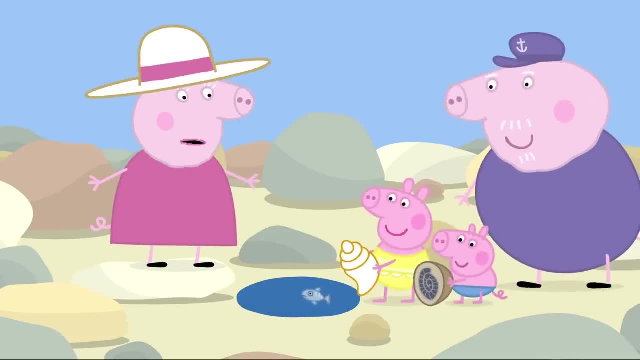 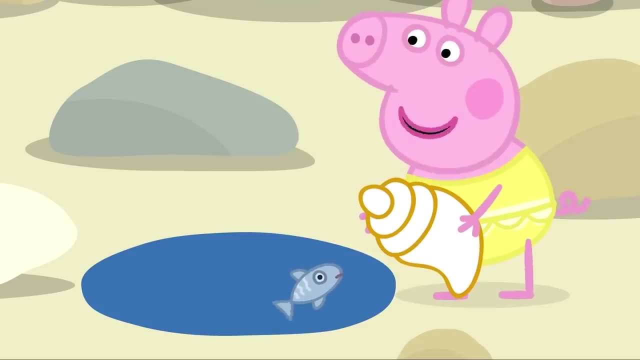 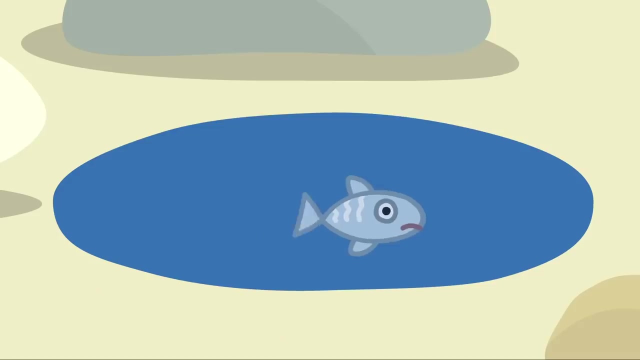 Where, Ooh, Poor little fish She's trapped. Oh Oh, The little fish says she wants to go back to the sea. Maybe you could use your bucket to rescue her. Yes, Peppa is rescuing the little fish in her bucket. 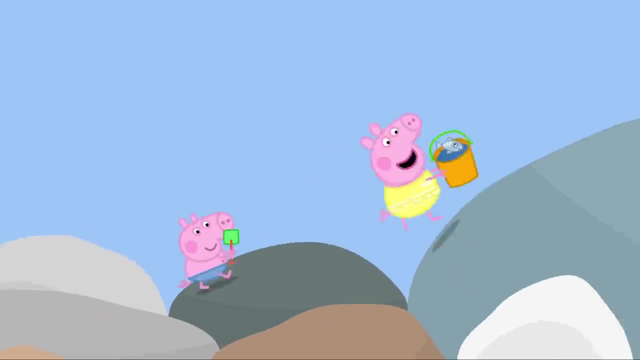 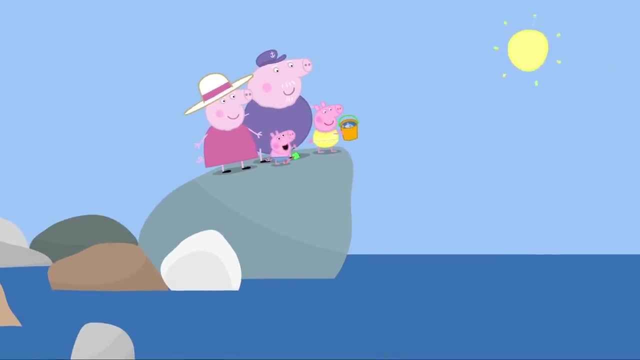 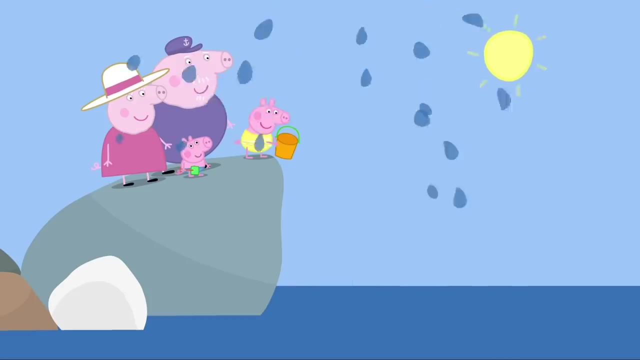 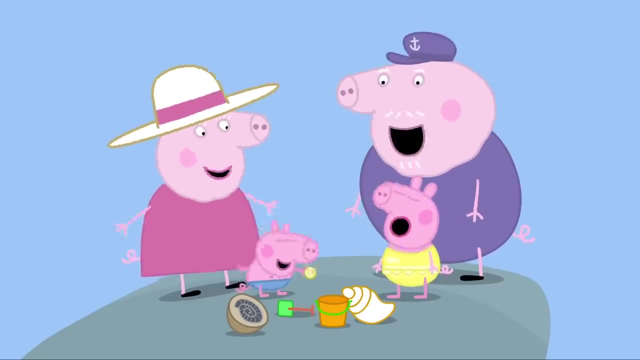 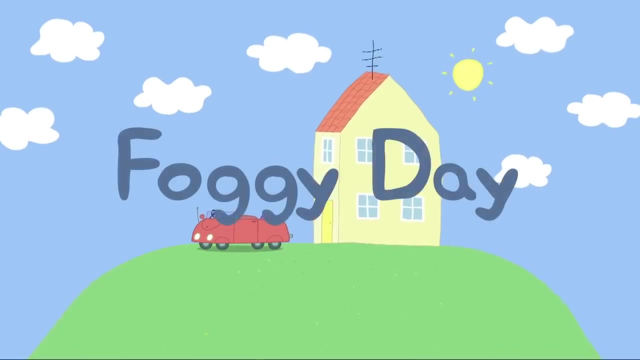 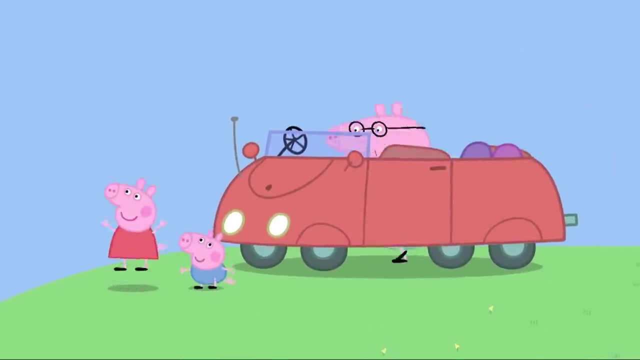 Don't worry, Mrs Fish, You'll soon be back with your friends. Bye bye, Mrs Fish, Bye, bye. Oh, I love rock pools. Foggy day: Peppa and George are going to the playground today. Should we drive to the playground? 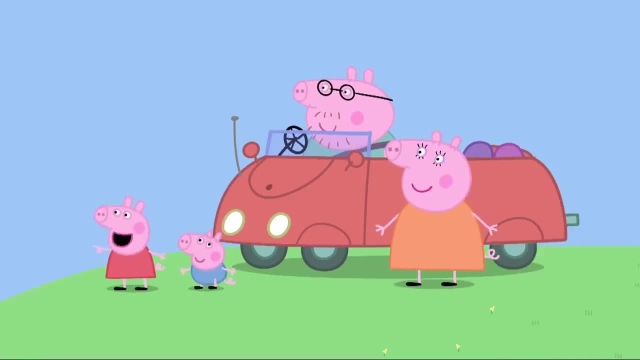 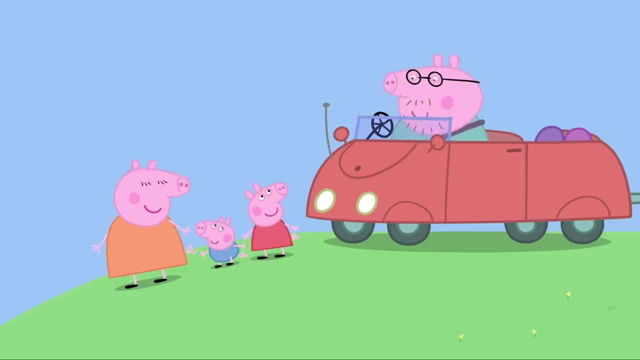 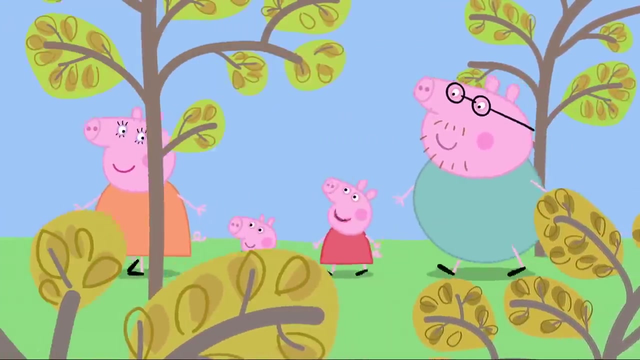 No, let's walk. Look, it's just over there. The playground is quite close. OK, let's walk. This way, everyone, We're going to the playground, We're going to the playground, We're going to the playground. 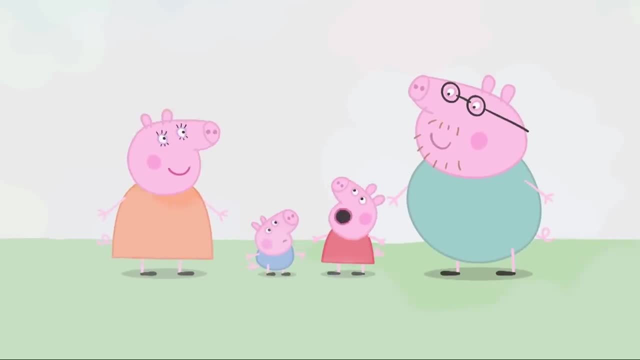 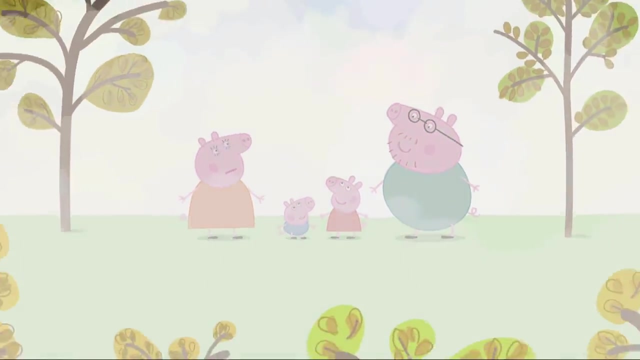 Oh, Where has the sky gone? Don't worry, Peppa, It's just fog. What's fog? Fog is a cloud that is on the ground instead of in the sky. Ooh, It's very thick fog. I can't see a thing. 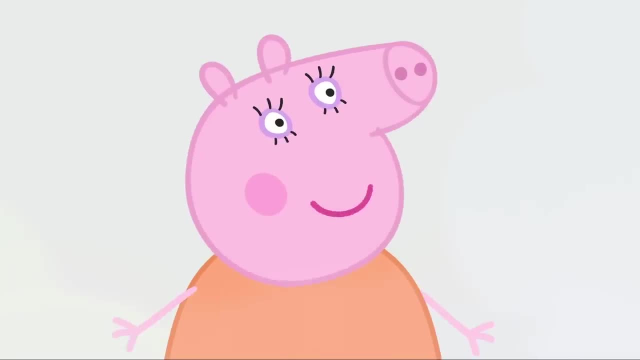 Hmm, Maybe we should go back home. Yes, we'll go to the playground another day. Aw, It is too foggy to find the playground, so Peppa and George have to go back home. Now, which way is home? 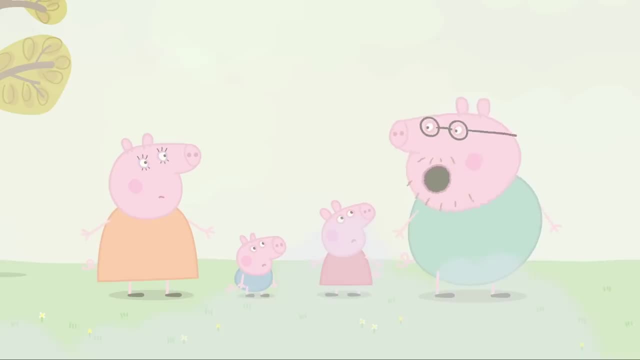 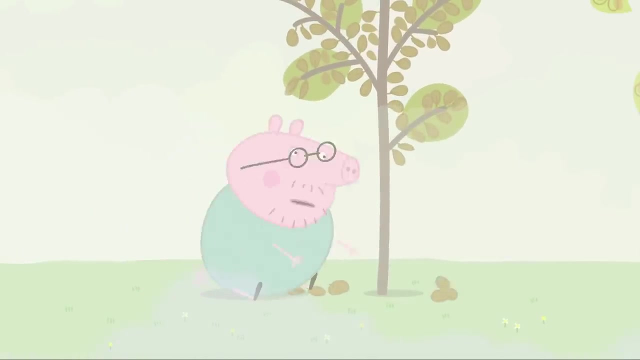 Are we lost, Daddy Pig? Oh, don't worry, I know exactly where we are This way. Ooh, Who put that tree there? Daddy Pig has walked into a tree. Are you OK, Daddy Pig? Yes, I'm fine. 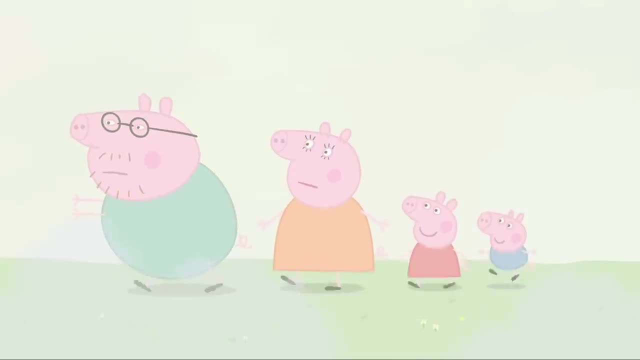 This way. Daddy Pig, do you know where you're going? Yes, of course I do. I don't think we'll ever find our house. I don't think we'll ever find our house. I don't think we'll ever find our house again. 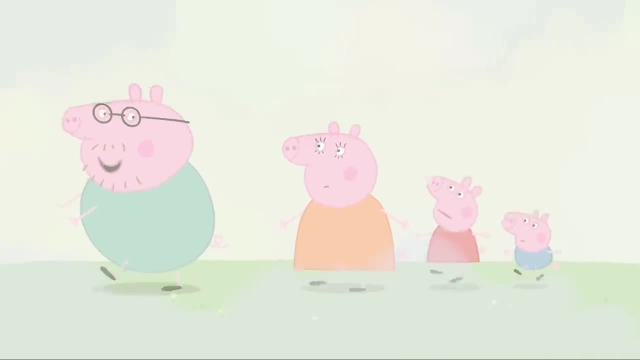 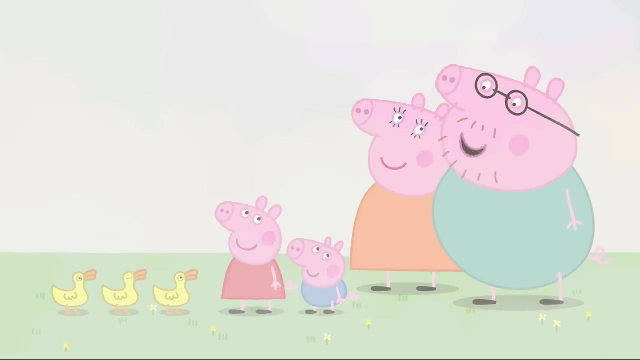 I'm sure we will, Peppa. We're only in our garden. Oh, it's the ducks. Hello, Mrs Duck, Have you lost your pond? We're lost too. We are not lost. I know exactly where we are. 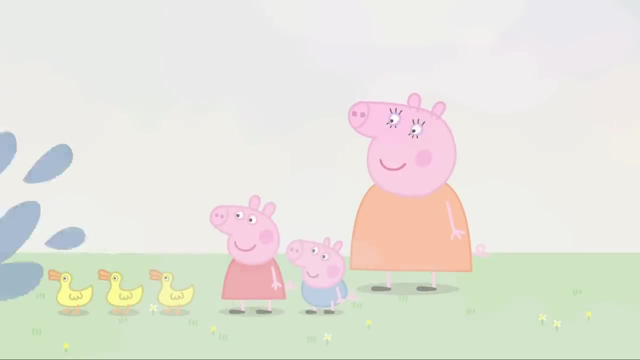 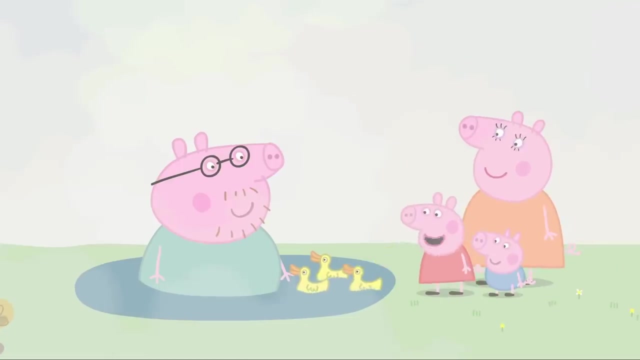 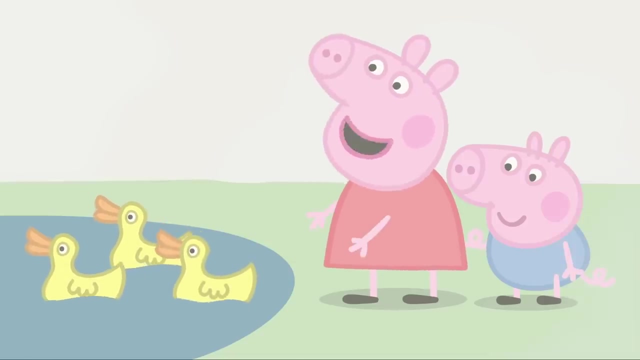 See you later, ducks, Good luck finding your pond. Ooh Ooh, Daddy Pig has found the duck pond. That's lucky. Yes, What a stroke of luck, Daddy. Mrs Duck says: thank you, You're most welcome, Mrs Duck. 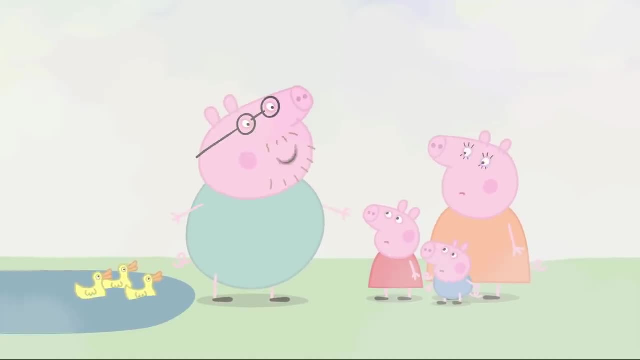 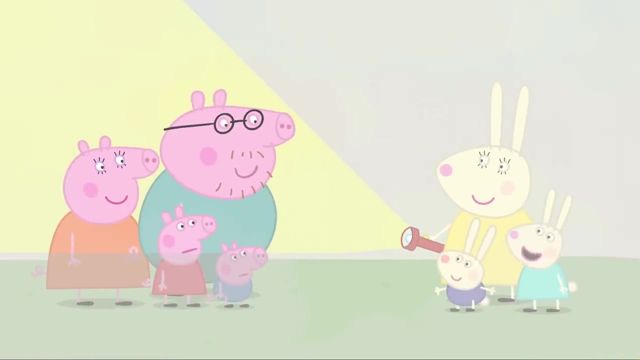 Now let's find our house. I'm sure it's this way. Hello, Did you hear something? Yes, I thought I heard someone say: Hello, It's Mummy Rabbit with Rebecca and Richard Squeak. Hello, Peppa. 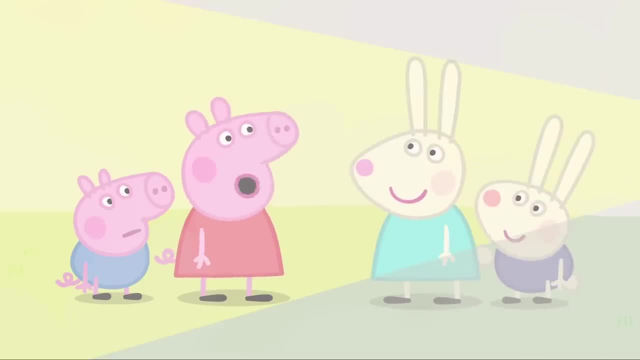 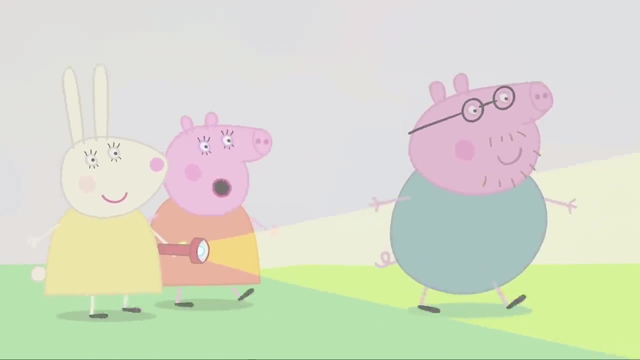 We're lost. Hello Rebecca, We're lost too. We wanted to go to the playground, So did we, But it's too foggy to get there. Come on, everyone Back to our house until the fog clears. Daddy Pig, do you know where you're going? 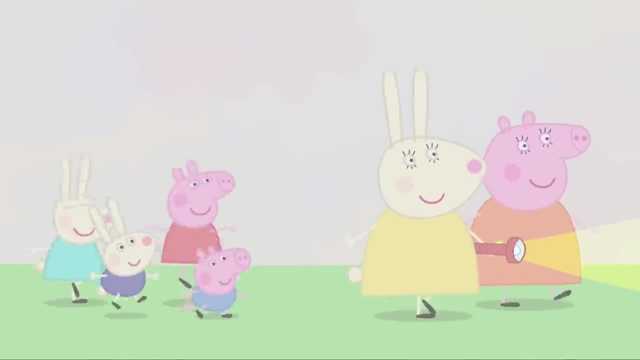 Yes, of course I do This way. Yes, Daddy Pig. Aha, I've found our little hill. We'll soon be home. Hooray, Our house should be just about here. Oh, Daddy Pig has found a ladder. 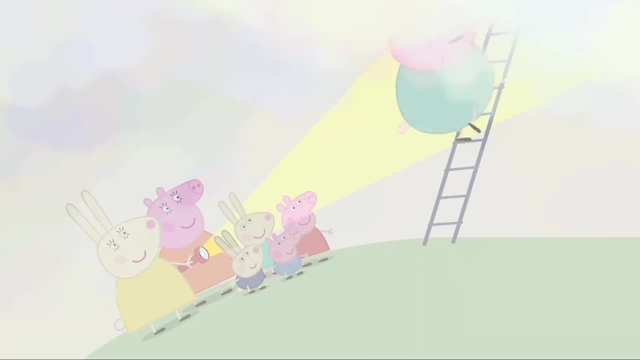 That's strange. We don't have a ladder in our garden. Goodness me, Can you see where we are, Daddy Pig? Yes, I can. Ho, ho, ho, ho, Daddy, Where are we? Why don't you have a look? 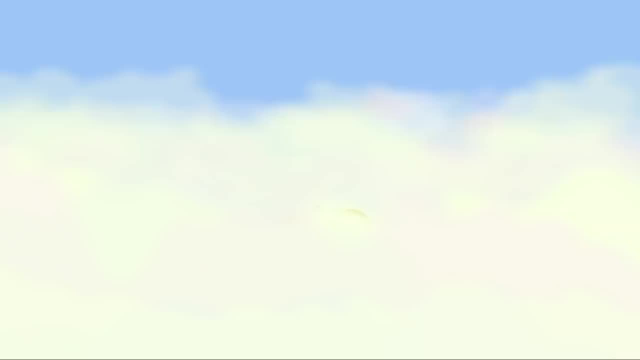 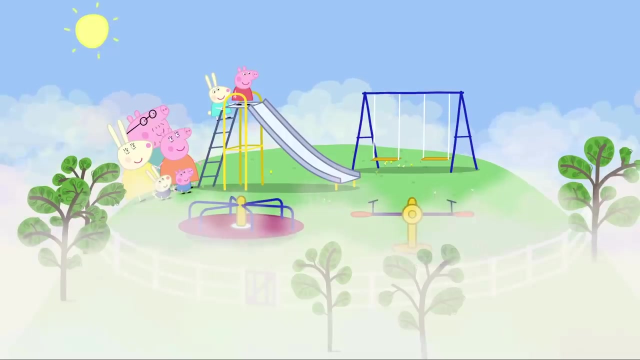 Okay, Wow, Wow, I can see everything again. The fog is going away. We're at the playground, Hooray, Whee. We're at the playground. We're at the playground, Whee, Ha, ha, ha ha. 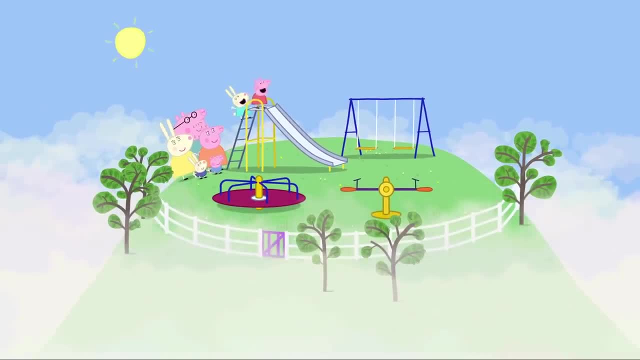 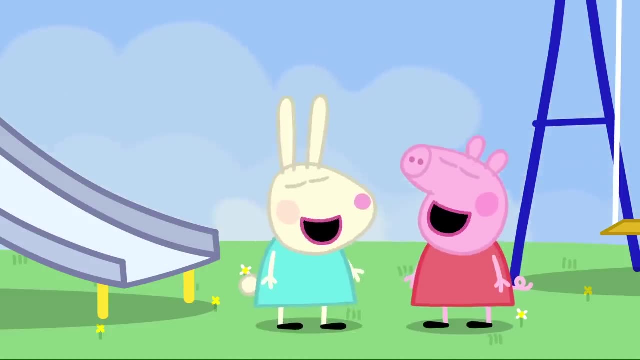 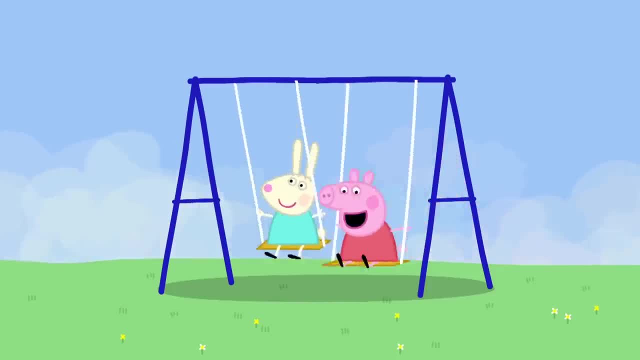 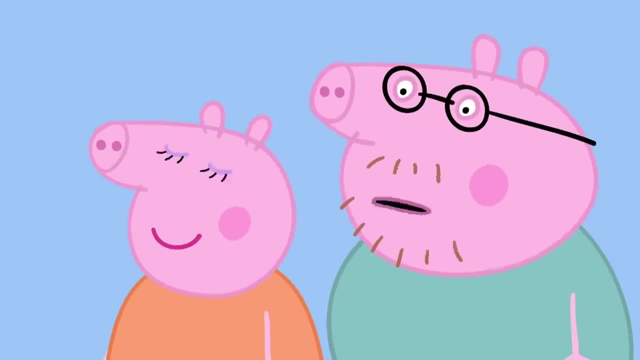 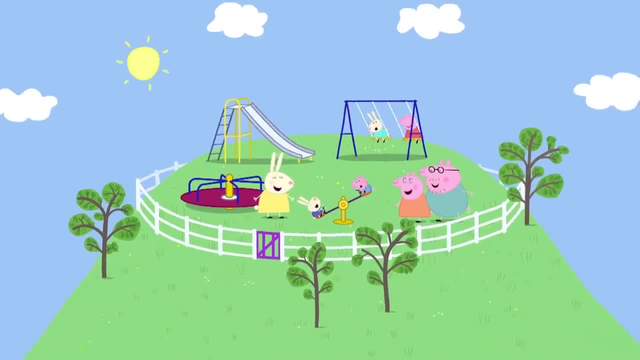 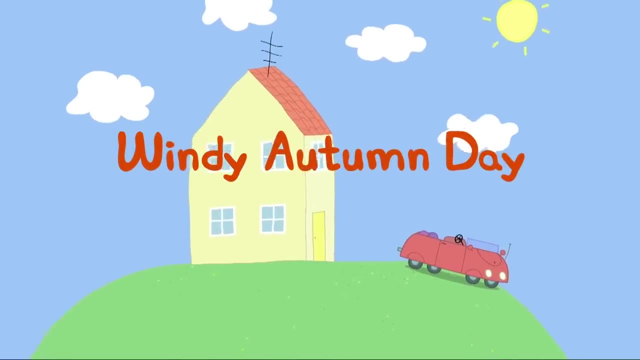 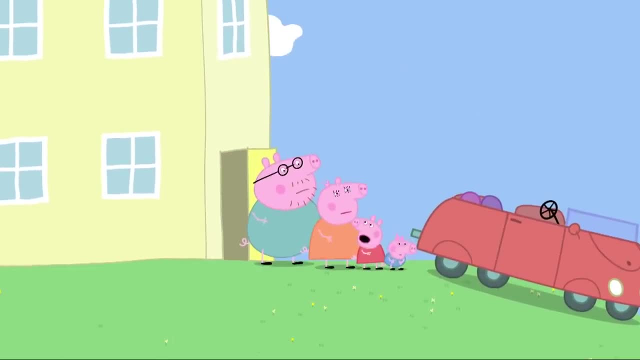 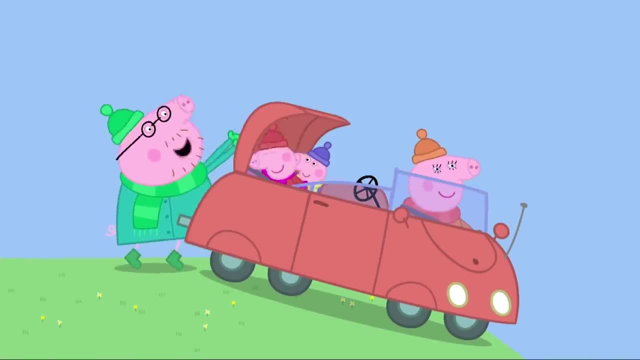 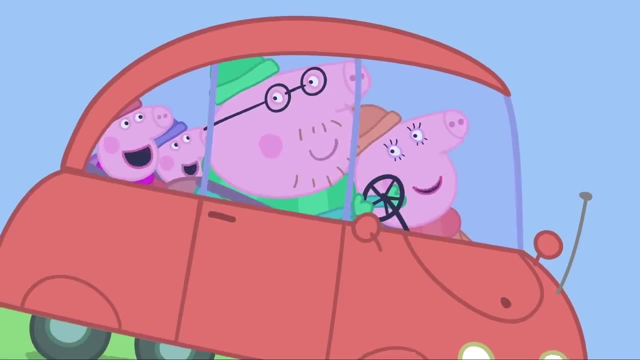 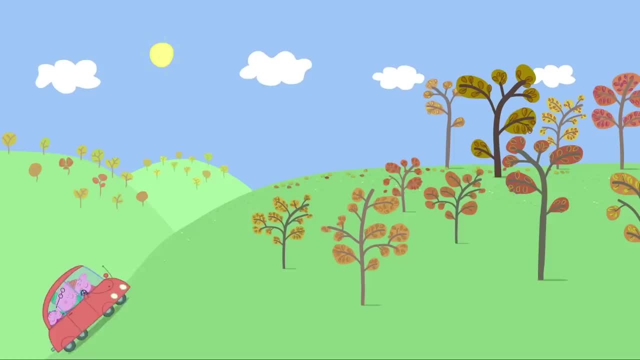 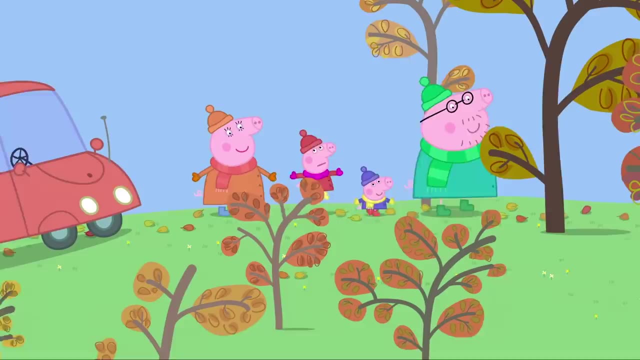 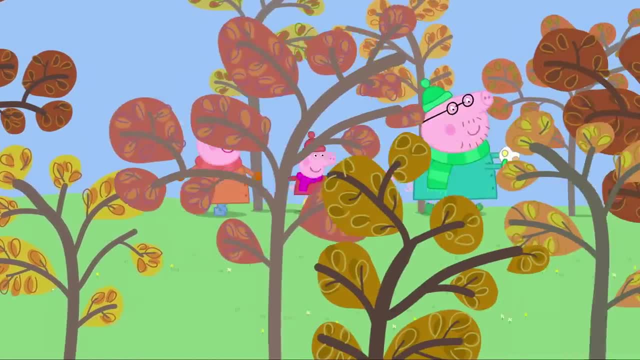 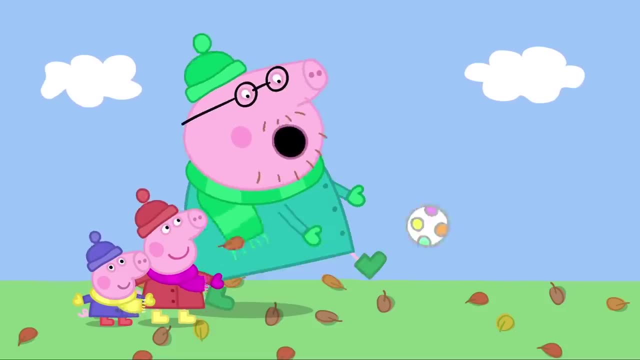 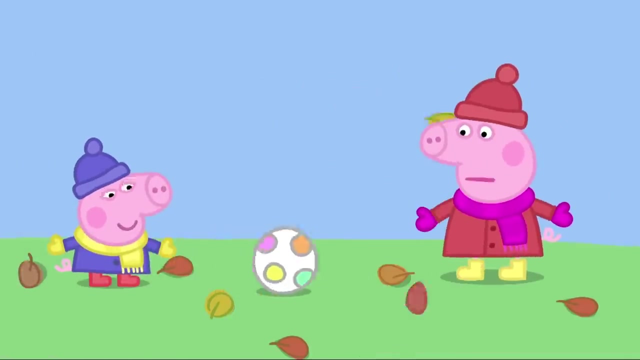 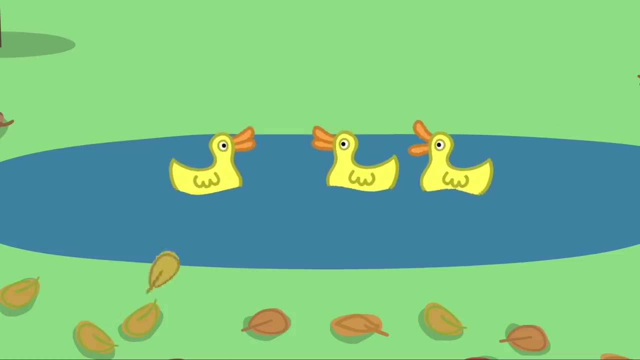 In the autumn it gets a bit colder and the leaves change colour. It's quite windy. Let's play a game to keep warm My turn. Oh, it's not meant to go that way. The wind is blowing the ball along. The ball is in the pond. 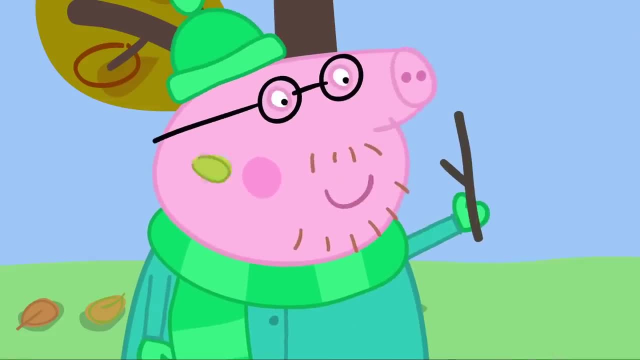 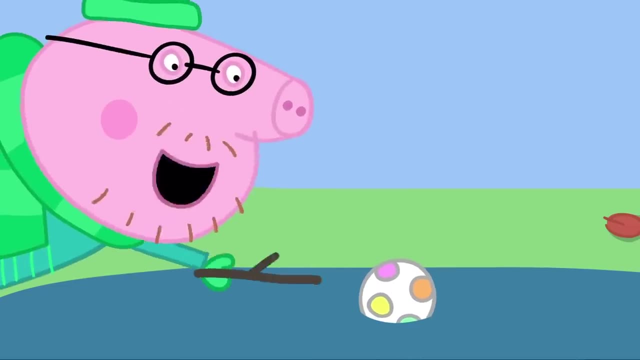 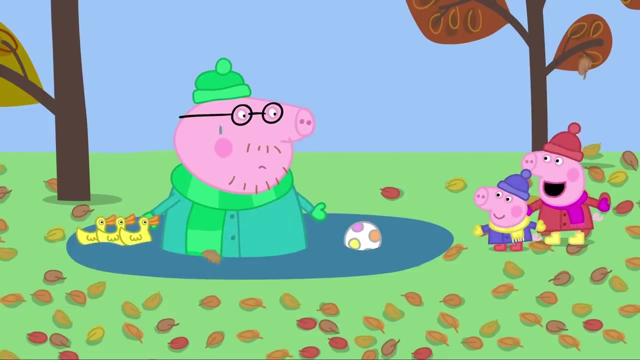 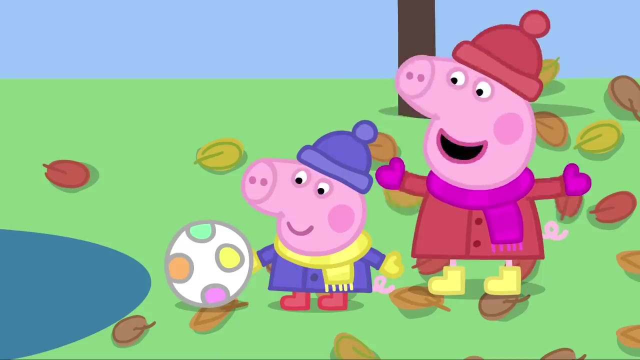 I'll just use this stick to reach it Just a bit further. Daddy, Be careful. Daddy Pig, Don't worry, I've almost got it. Daddy, is the water cold A little bit? The wind has blown the ball out of the pond, That's lucky. 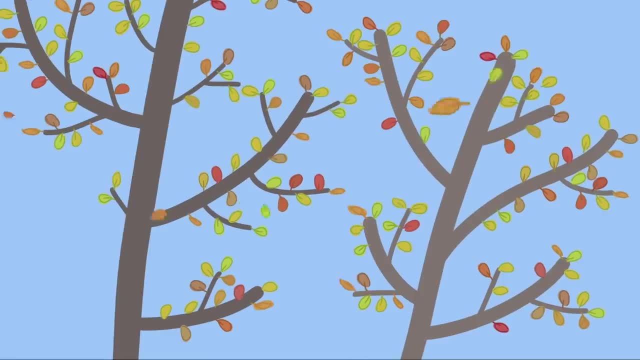 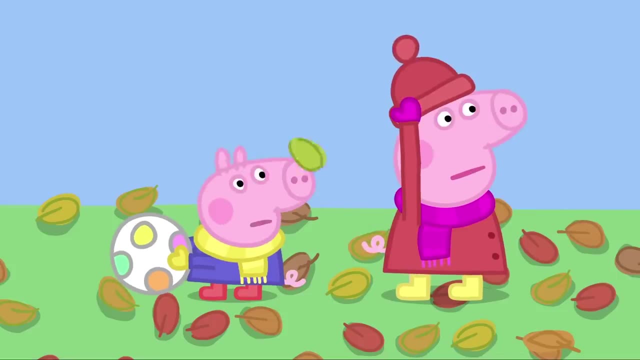 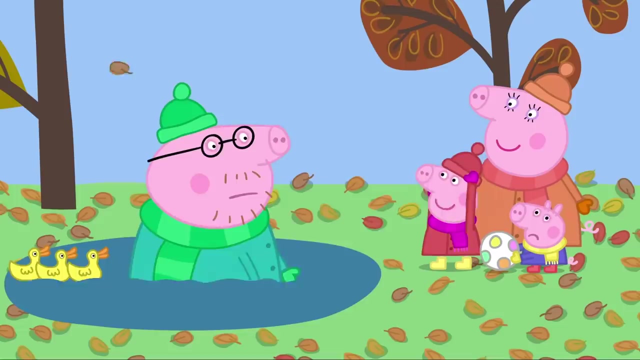 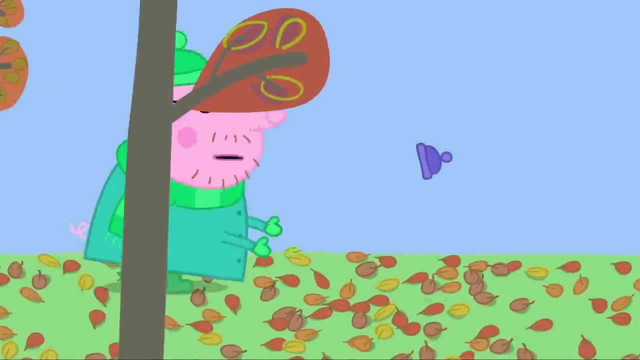 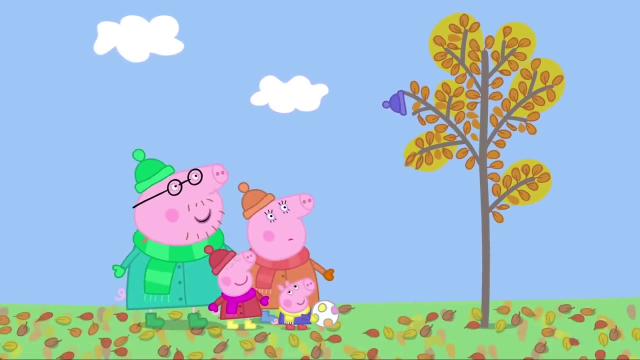 Yes, what a stroke of luck. It's getting even windier. Hold on to your hats. No, the wind has blown George's hat off. Don't worry, George. Daddy Pig will catch your hat Quick Daddy. Look, it's in that little tree. Hmm, I'll just climb up and get it. 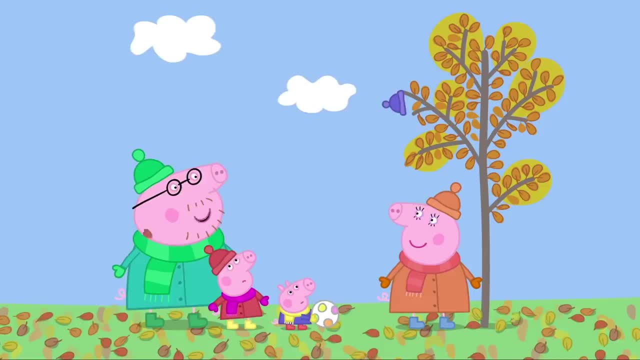 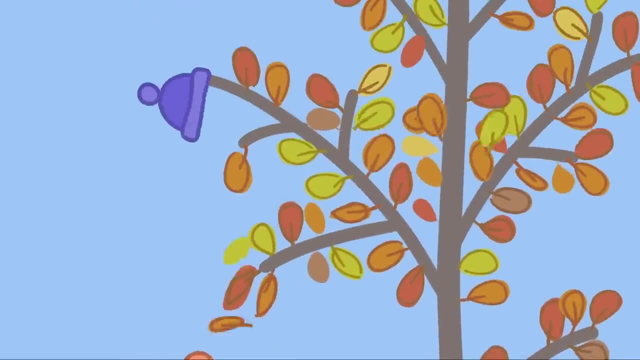 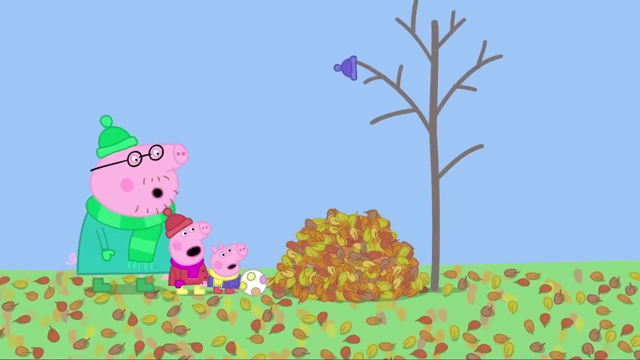 The tree is much too thin to take your weight, Daddy Pig. So how can we get George's hat Simple? I'll give the tree a little shake. Huh, maybe if I shake it a bit harder. Oh Oh, I thought that sort of thing only happened to me. 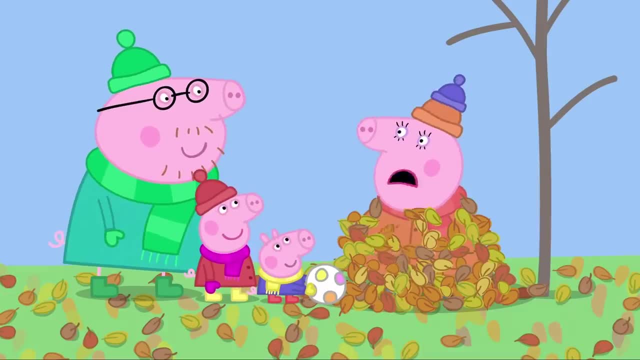 I thought that sort of thing only happened to me. I thought that sort of thing only happened to me. It's not funny. It is a bit funny, Mummy. I suppose it is a bit funny. Where's George's hat? It's on your head. Here's your hat, George. 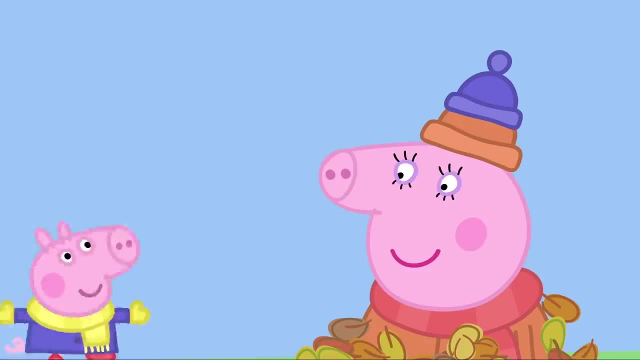 Hold on to it. this time The wind is blowing all the leaves off the trees. Look at me. I'm leaning into the wind. The wind is strong enough to hold Peppa up to the tree. Peppa, Peppa, Peppa. 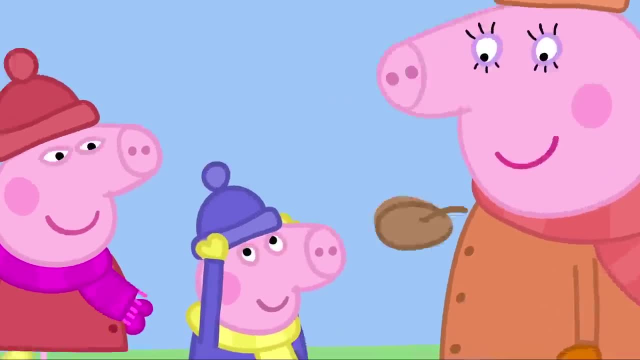 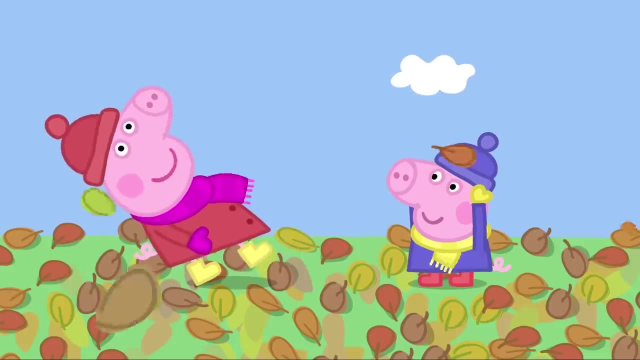 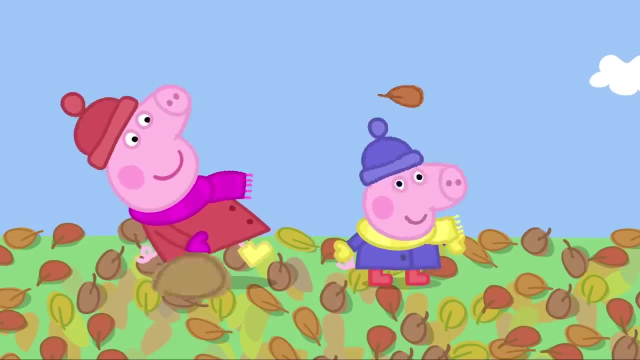 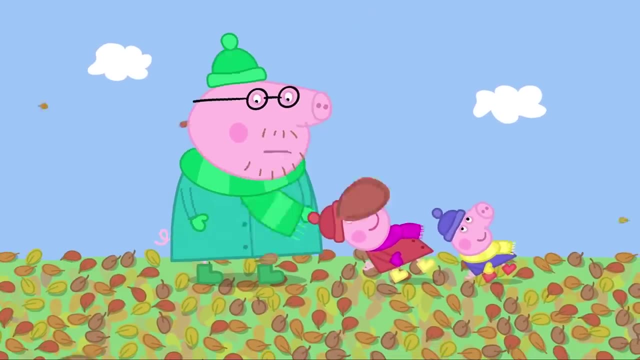 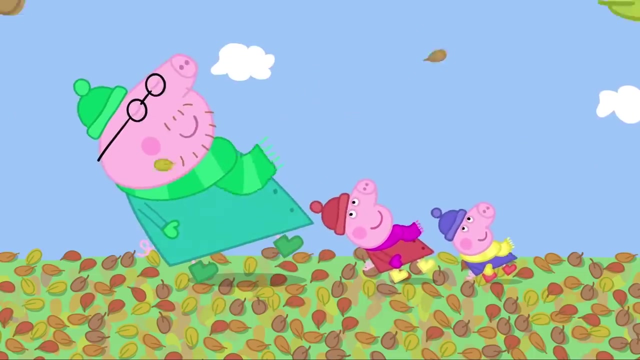 Peppa, Peppa, Peppa. The wind is strong enough to hold George up. Daddy, have a go, I'm a bit too heavy. Come on, Daddy, It's really fun. All right, The wind is strong enough to hold up Daddy Pig. 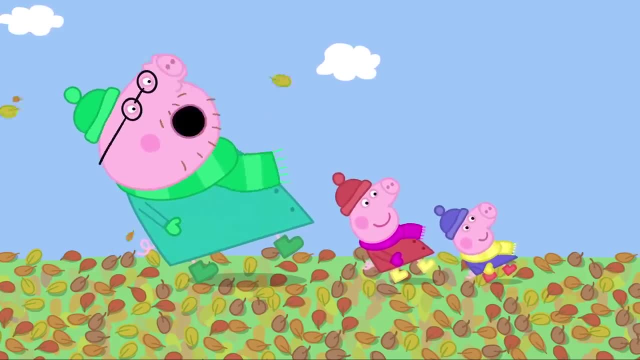 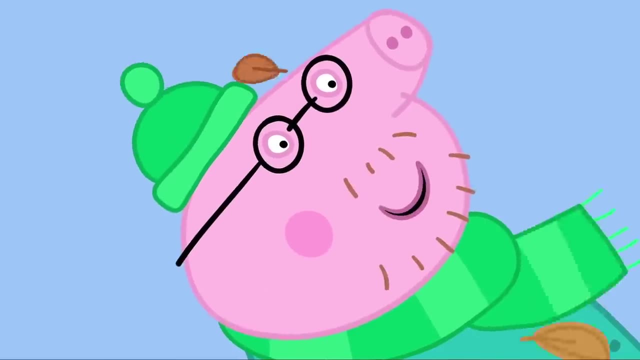 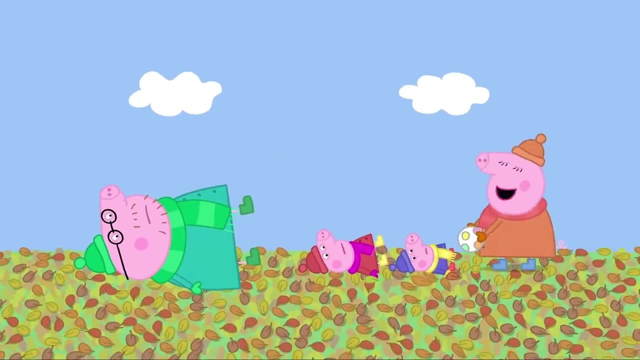 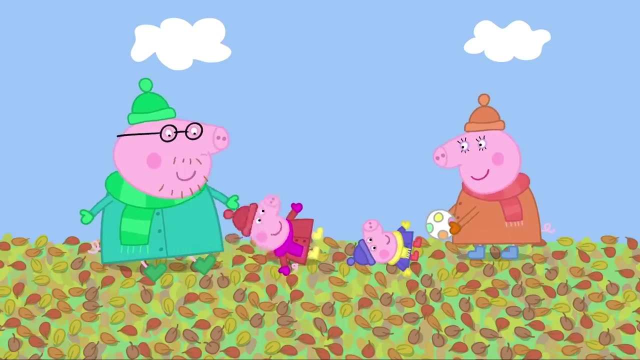 I say this is fun. Come on, Mummy Pig, give it a try. But if the wind stops I'll fall over. The wind won't just stop. Stop, The wind has stopped. It's not funny, It is a bit funny. Now the wind has stopped, what can we do? 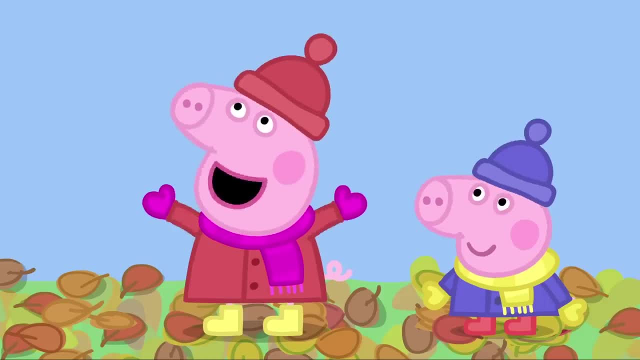 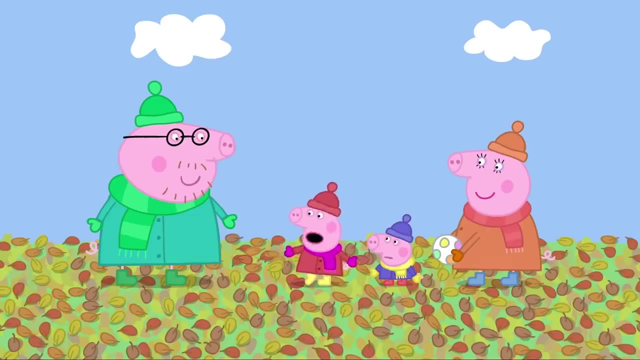 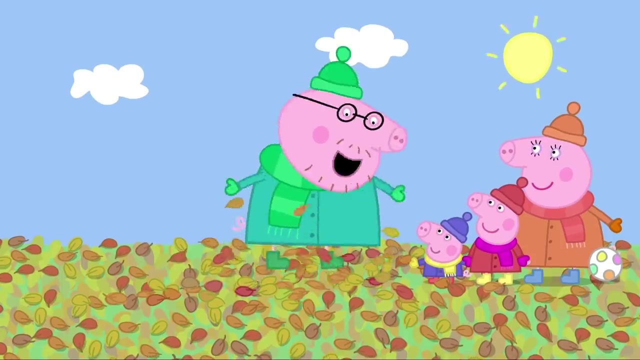 Hmm, What's your favourite game? Jumping up and down in muddy puddles. But there aren't any puddles, Just lots of boring dry leaves. And what do you do with dry leaves, I don't know? Jump up and down in them. 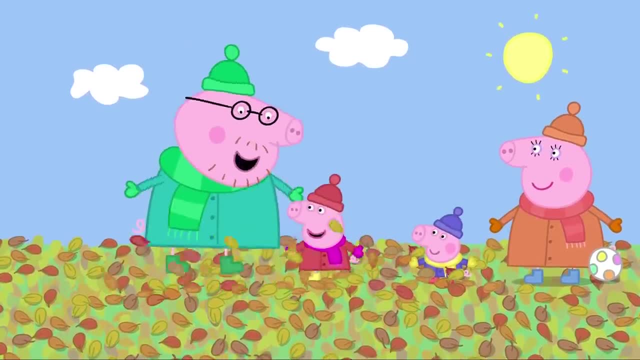 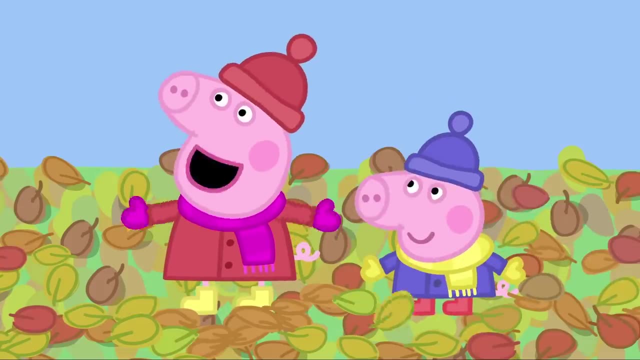 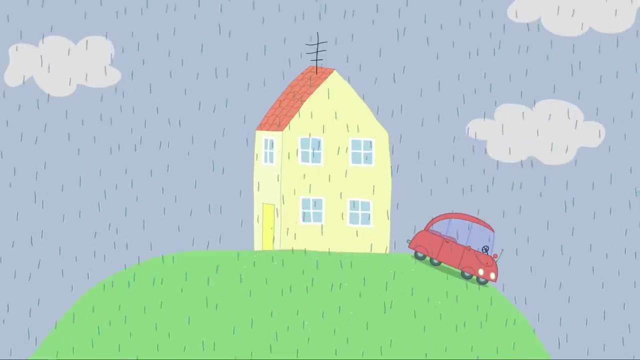 Daddy Pig loves jumping up and down in leaves. Peppa loves jumping up and down in leaves. Everyone loves jumping up and down in leaves. This is the best autumn day ever. George catches a cold. Today it is raining a little bit. 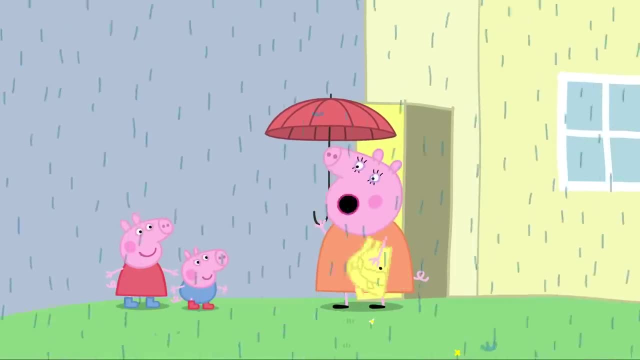 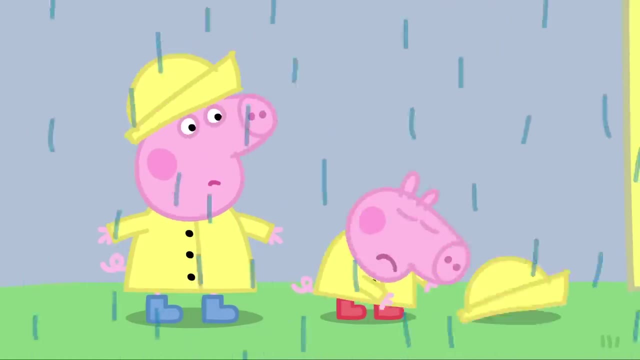 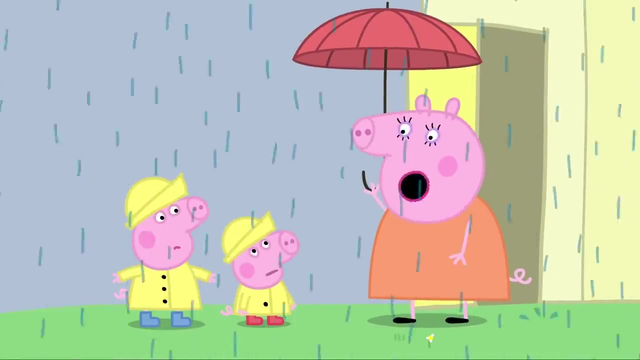 Peppa, George, put your rain clothes on When it rains. Peppa and George must wear their rain clothes. Yuck, George does not like wearing his rain hat. George, you must keep your hat on Why? Because you must keep dry. 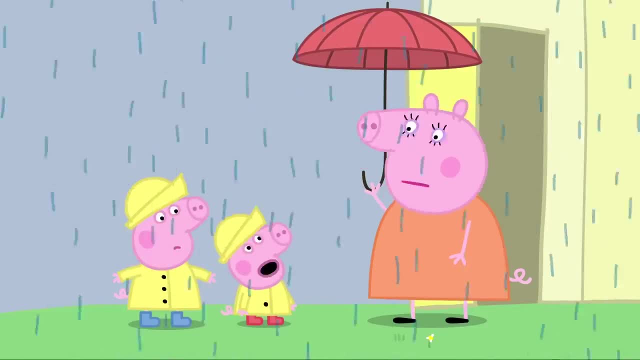 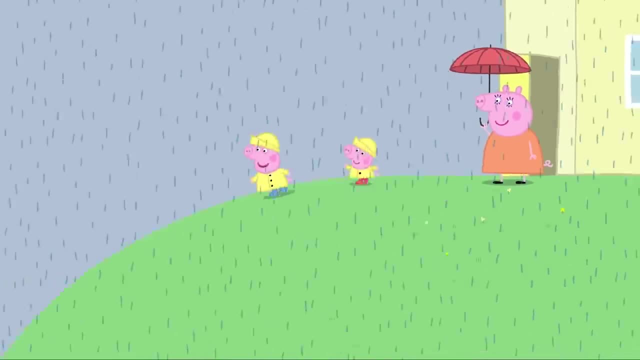 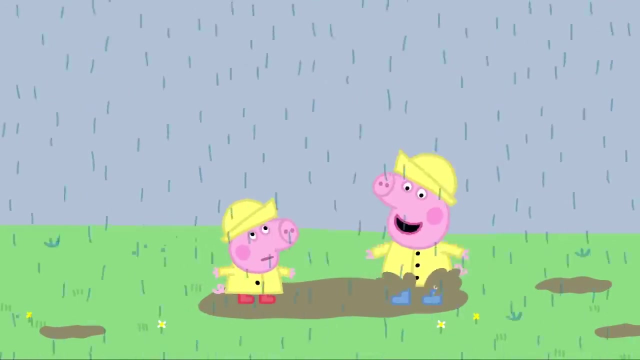 Why? Because you might catch a cold. Why, George, do you want to play in the garden? Then keep your hat on. Come on, George. Peppa and George are going to jump in muddy puddles. Yuck, George does not want to wear his rain hat. 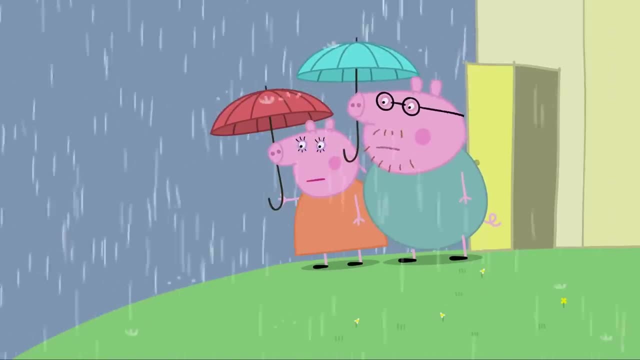 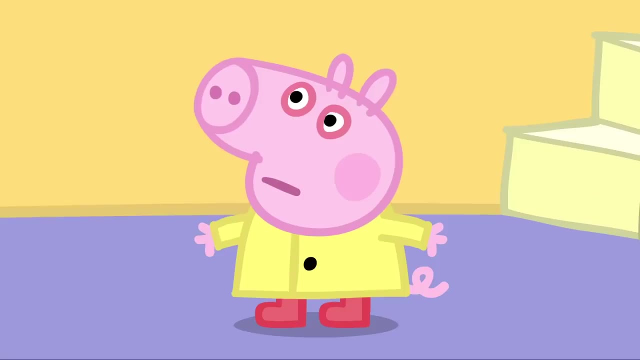 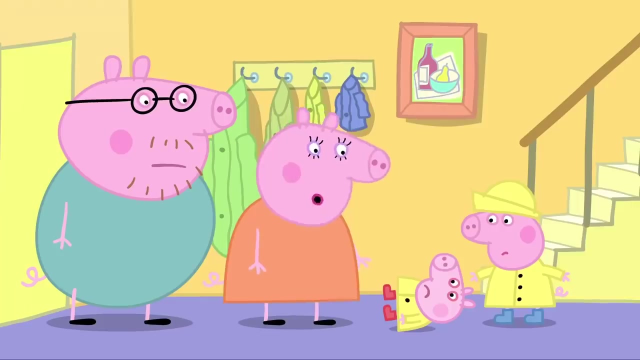 Peppa George, Come inside. The rain's too heavy to play in now. No, Oh, George, where's your hat? Achoo, George has caught a cold. Achoo, Oh, poor little George, You don't sound well. 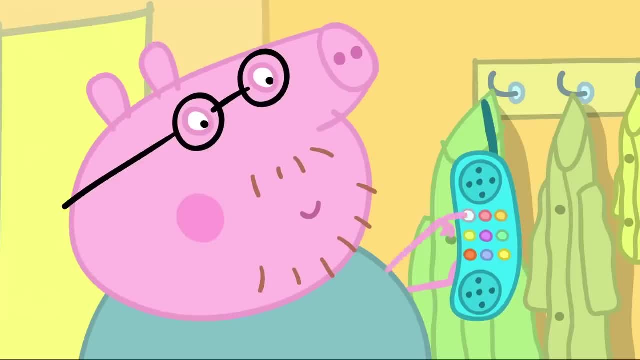 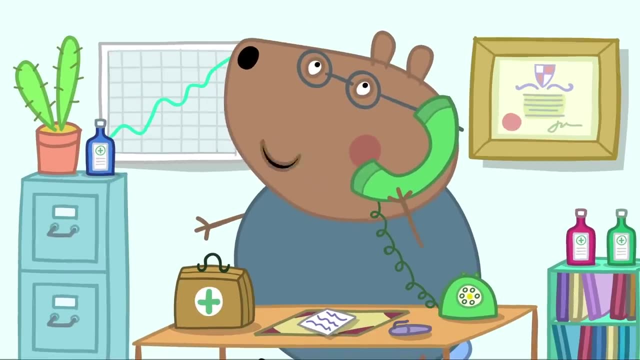 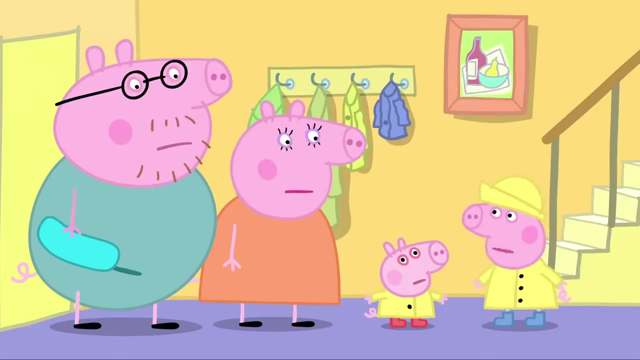 Don't worry, I'll ring Dr Brown Bear. Dr Brown Bear speaking. I see, Put George to bed and I'll be straight round. Thank you, Dr Brown Bear. Goodbye, Will George be taken to hospital and given medicine? No, George just has to go to bed. 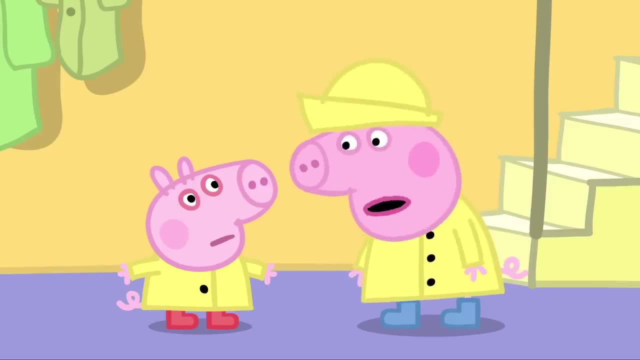 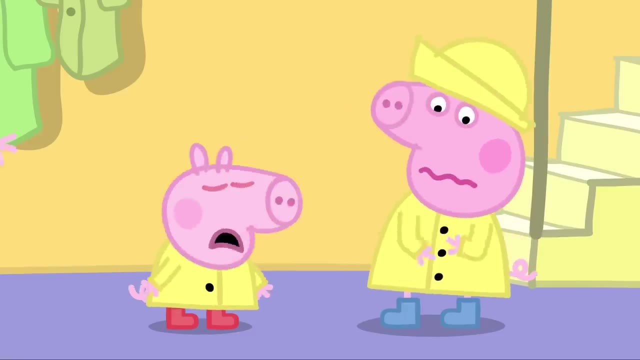 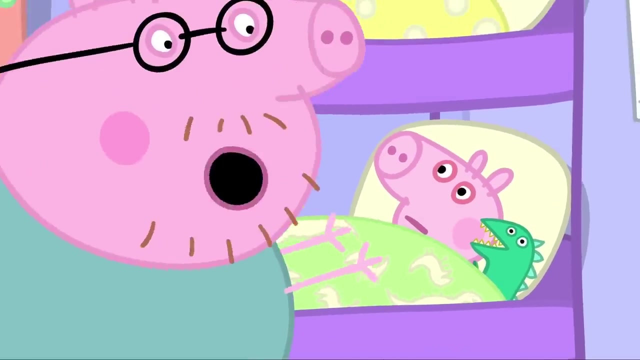 Oh, So George is not really properly ill. Achoo Eurgh, That's disgusting, Poor George. Let's get you straight to bed. George, you have to stay in bed for a bit. No, George does not want to stay in bed. 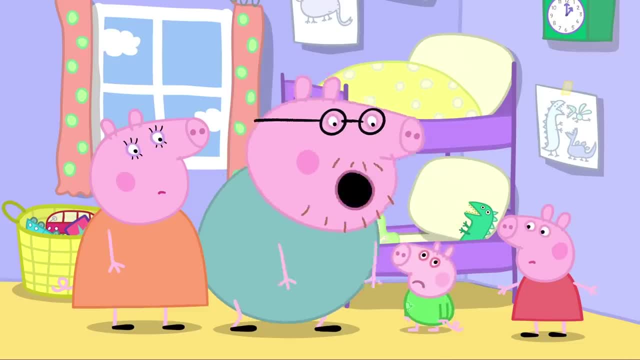 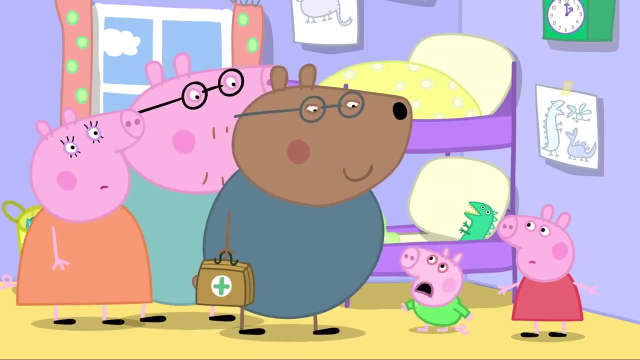 Achoo, George, you have to stay in bed until you are better. Why? Because you have to keep warm. Why, Er, because Dr Brown Bear says so. Hello, Where's my patient? Open wide and say aww. 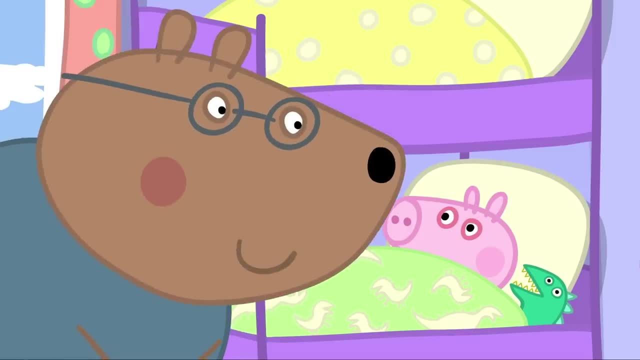 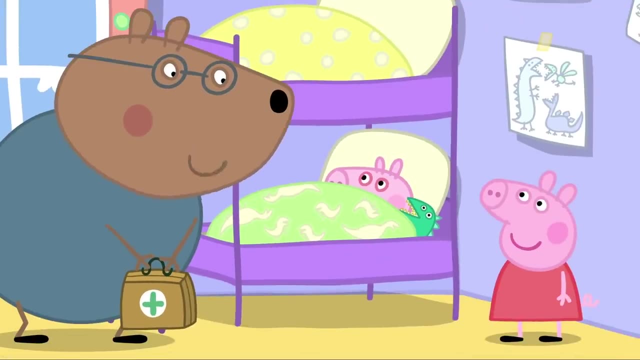 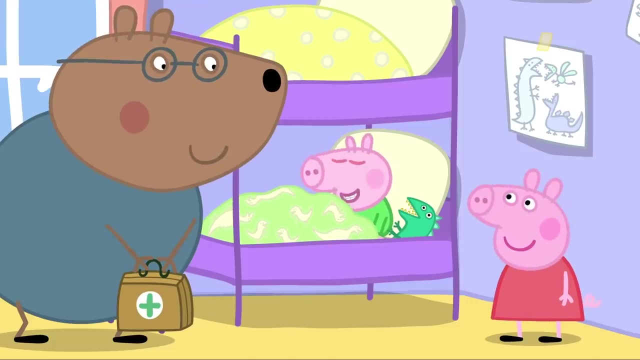 Achoo And say, aww, George is a little bit worried. Hmm, Peppa, you're big and brave. Can you show George how to say aww, Of course, Awww, Awww, Hmm, George has caught a cold. 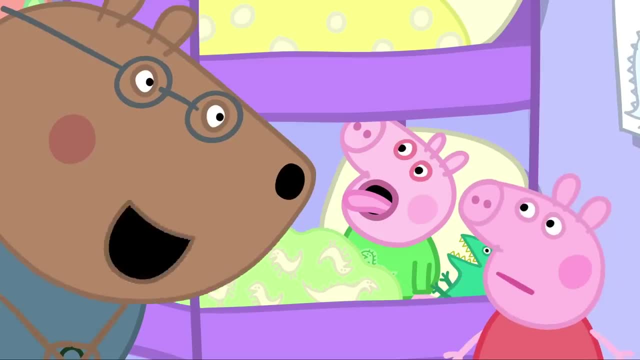 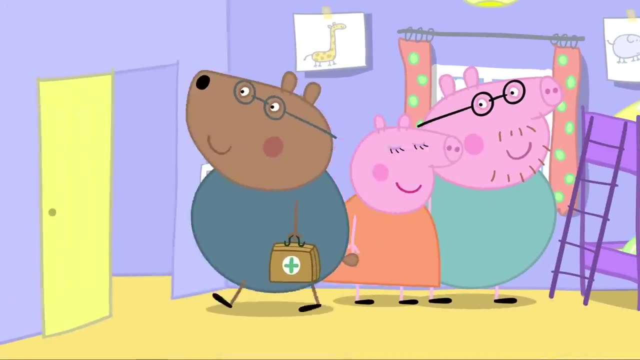 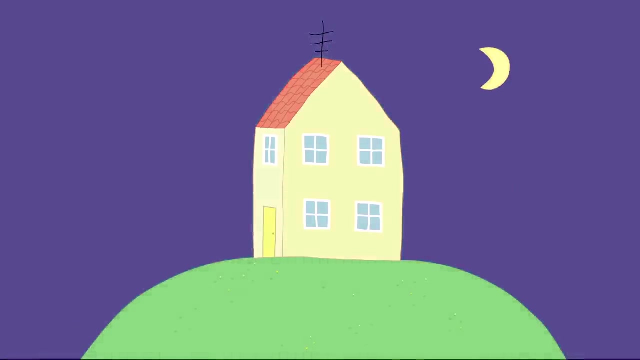 Does George need medicine? No, but he can have some nice warm milk at bedtime to help him sleep. Thank you, Dr Brown Bear, You're welcome. Goodbye, George has been in bed all day. Now it is Peppa's bedtime. 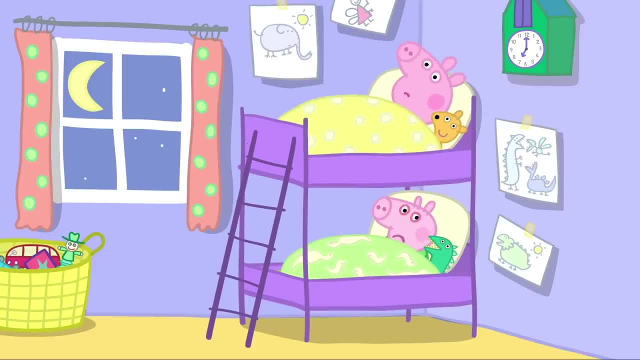 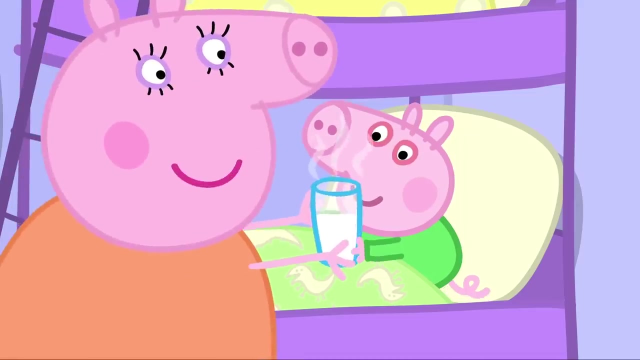 George, are you better? Achoo, George is not better. Achoo George, please don't sneeze so loudly. This is impossible, George. here's some nice warm milk. Here's some nice warm milk to help you sleep. 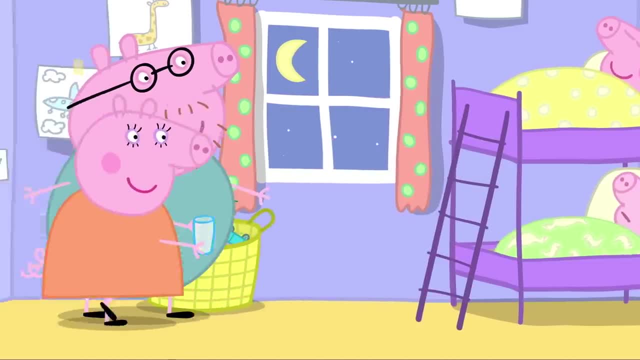 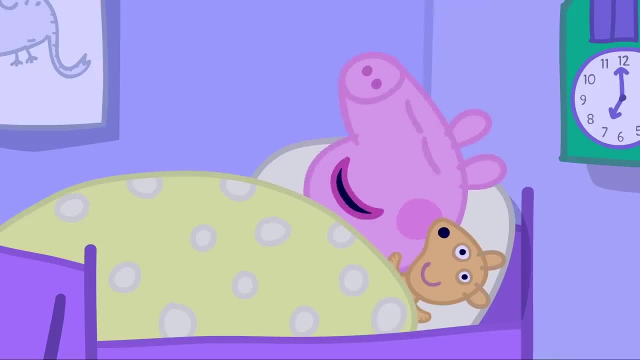 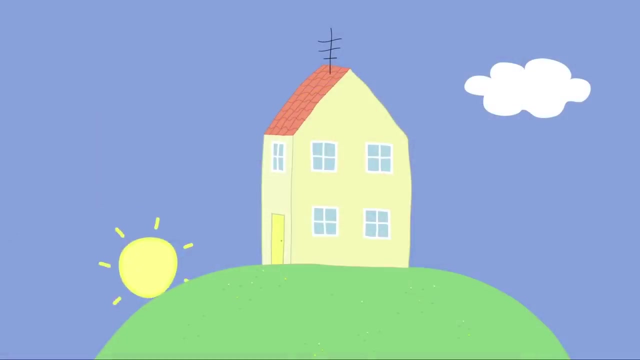 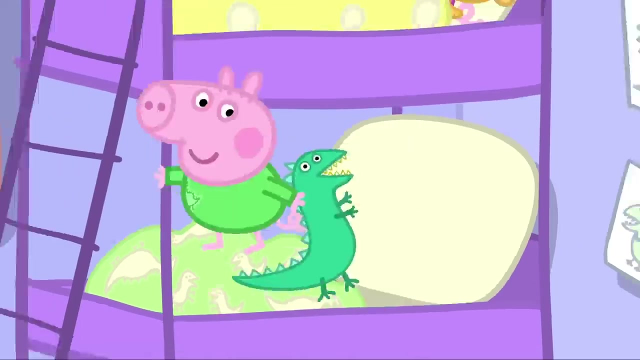 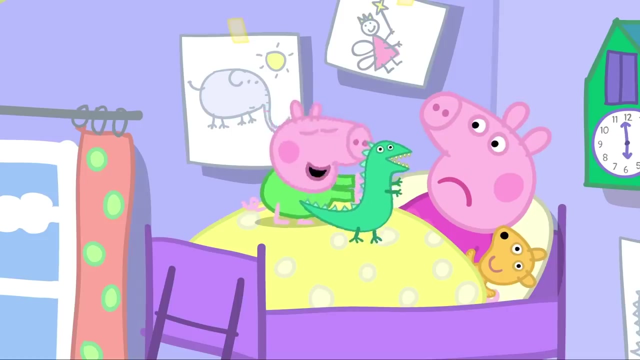 The warm milk makes George feel very, very sleepy. Good night, my little piggies. It's so nice and quiet. It is morning. George has slept very well. George is better. Come on everyone. It's a lovely sunny day. 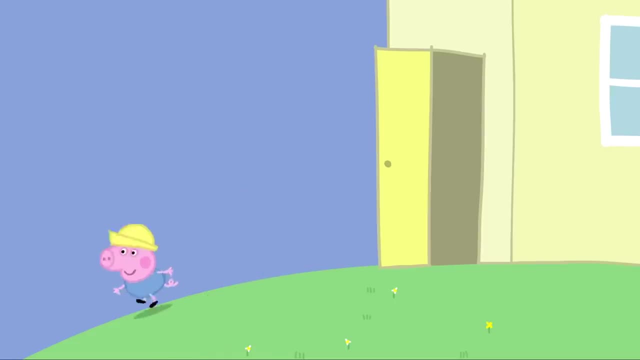 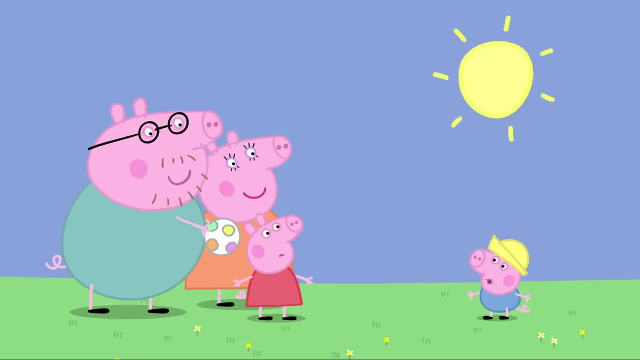 George is wearing his rain hat. He doesn't want to catch another cold. Oh, George, you don't need to wear your hat. Why? Because it's hot and sunny. Why, George, can you stop saying why all the time? 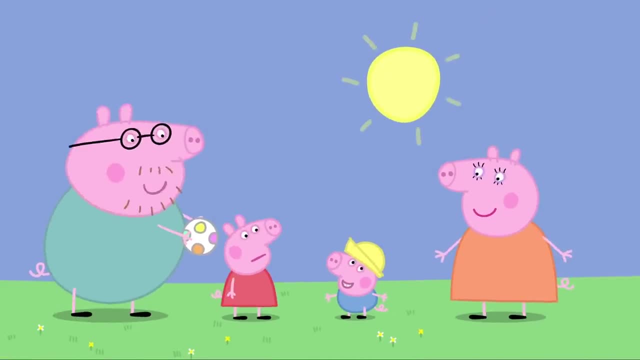 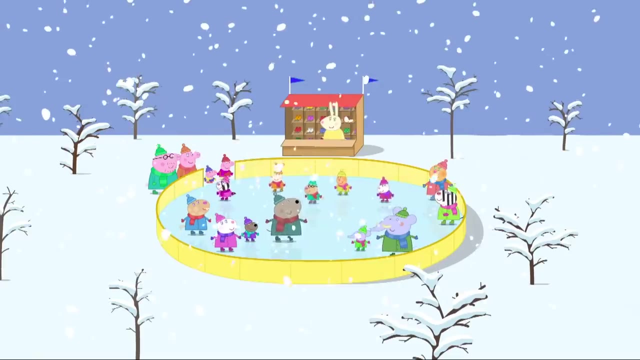 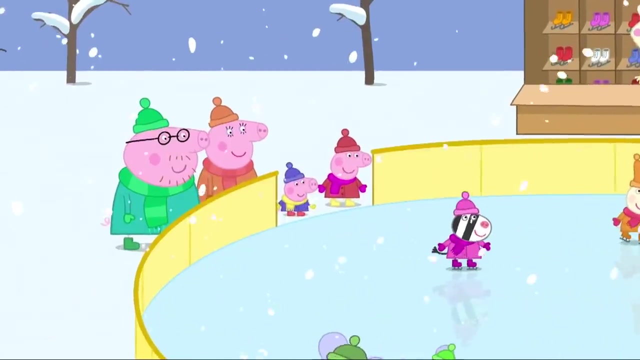 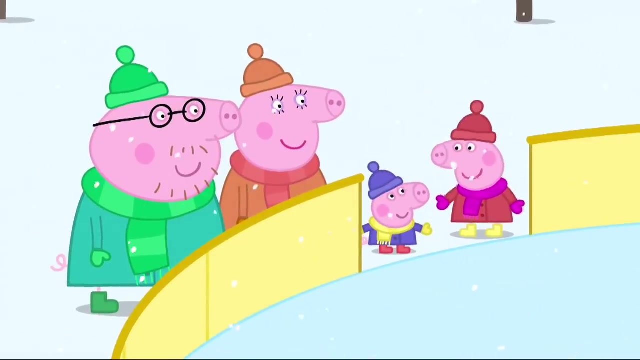 Why George certainly is better Ice skating. Peppa and her family are going ice skating today. This will be fun. Peppa and George have never been ice skating before. Now, George, you won't be very good at ice skating. 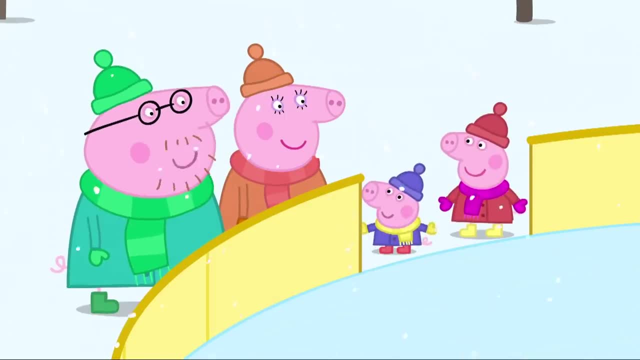 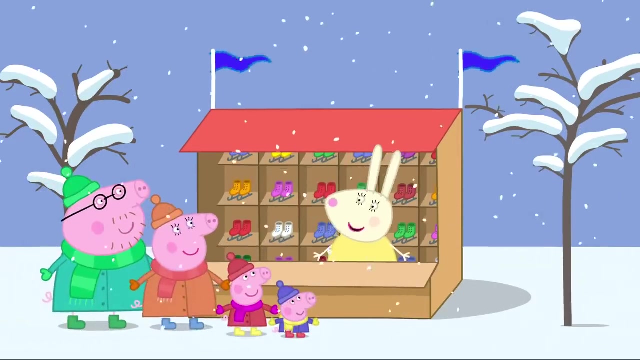 So just do what I do. I'm sure we'll all be very good- Yes, especially me. First, we need some skates. At the ice rink, everyone wears skates. Hello, Miss Rabbit, Hello Mummy Pig. 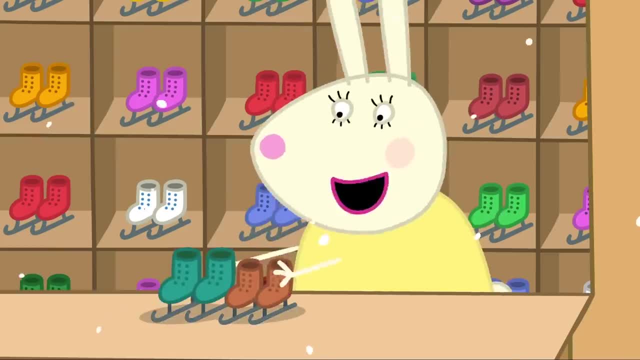 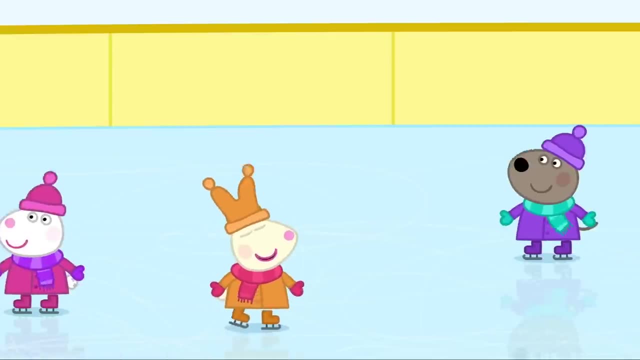 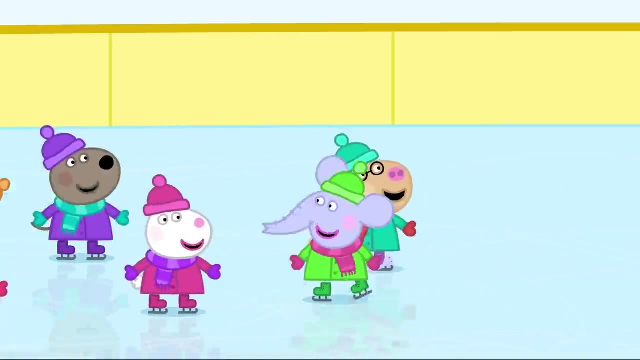 We'd like to hire some skates please. There you go, Thank you, Happy skating. Here are Susie Sheep, Rebecca Rabbit, Danny Dog, Zoe Zebra, Candy Cat, Emily Elephant and Pedro Pony. Peppa's friends can ice skate very well. 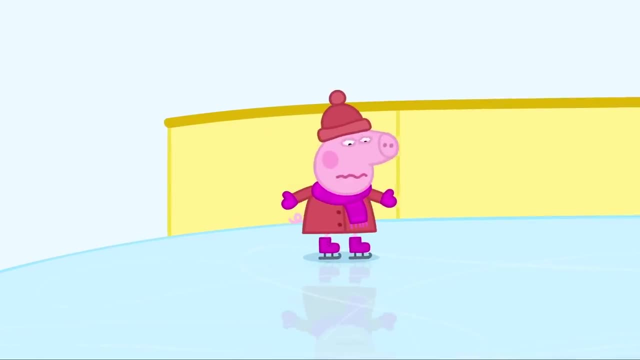 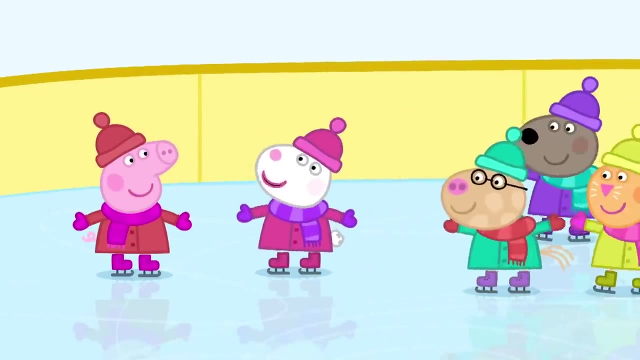 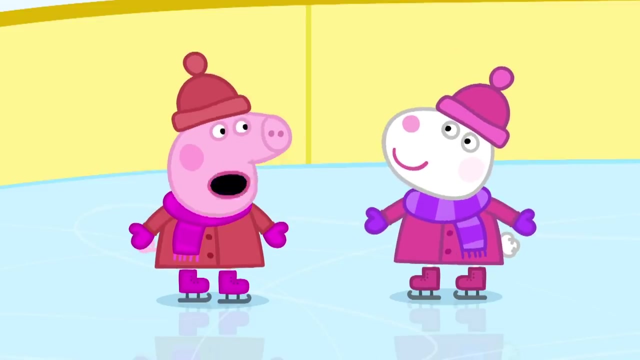 Peppa wants to ice skate too. Hello everyone, Hello, Peppa, Is this your first time skating? Yes, Shall I show you how to skate. No, thank you, Susie, I'm sure I can already do it. 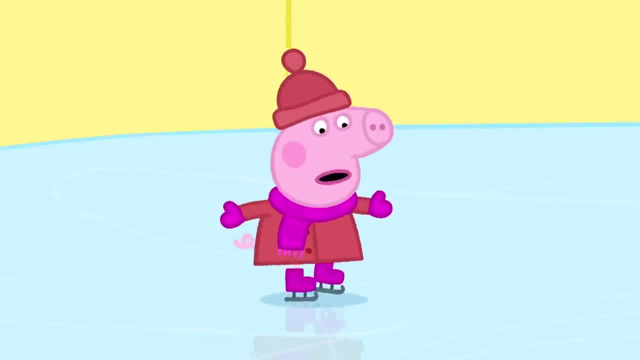 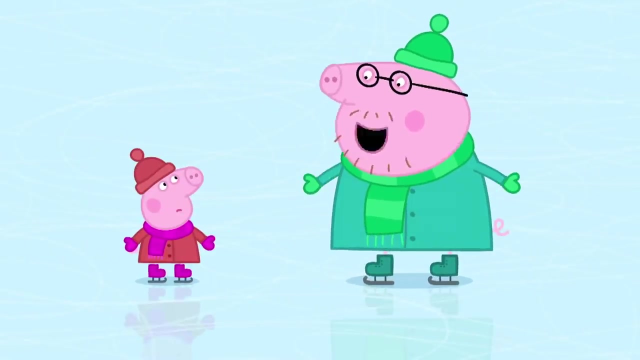 Okay, come on then. This is impossible. I don't want to do ice skating anymore. Don't worry, Peppa, Everyone falls over when they ice skate. Even I fall over. Watch this, Oops-a-daisy, Ho-ho. 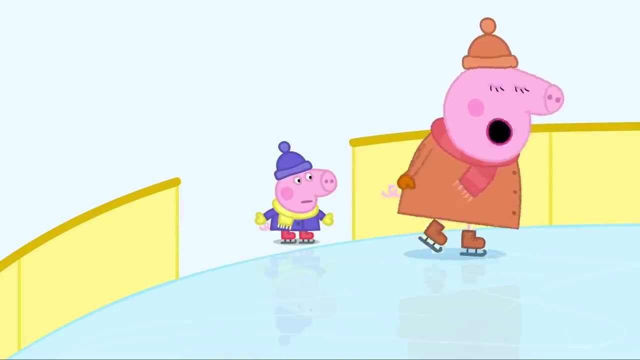 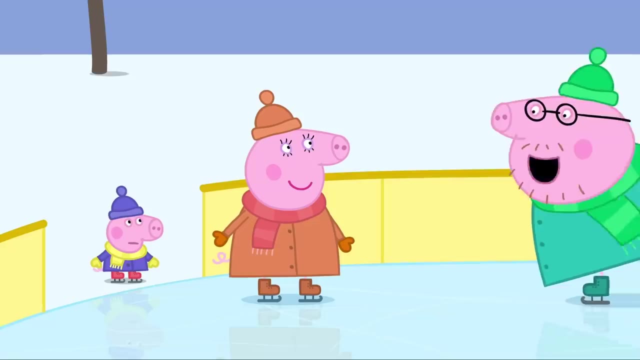 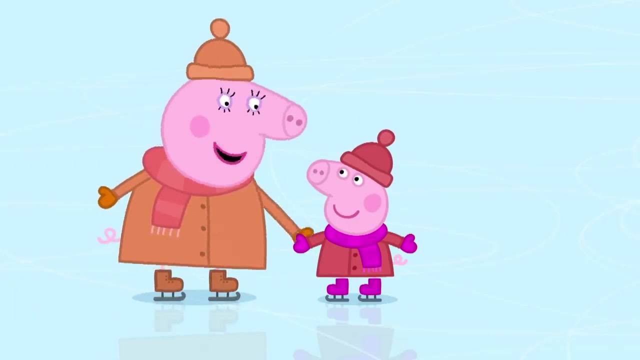 Silly Daddy. George, would you like to skate? No, George has never ice skated before and he is a bit worried. I'll look after George while you teach Peppa how to skate. Skating is easy, Peppa. 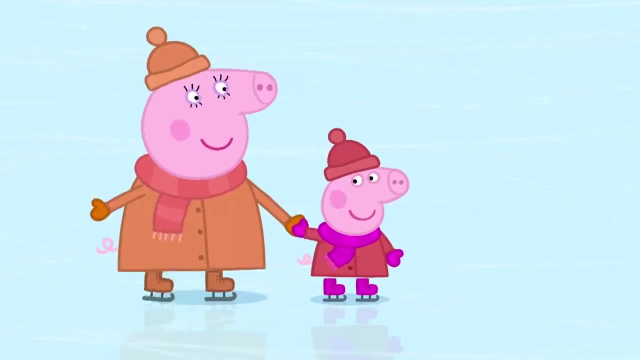 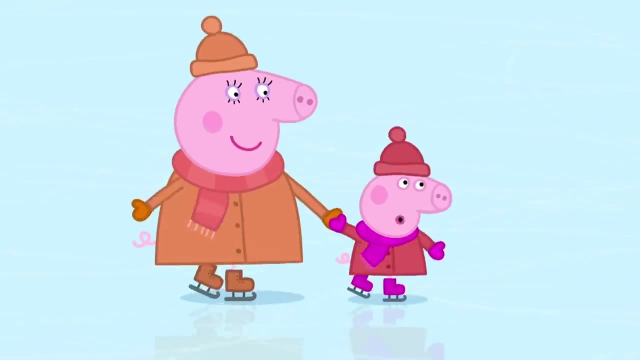 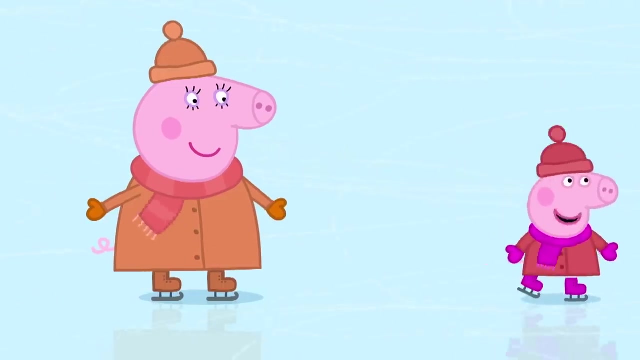 Just push with your feet and glide- Push, push glide See: Push push glide, Push, push glide. This is easy. I can do it on my own now, Mummy, Push, push glide, Push, push glide. 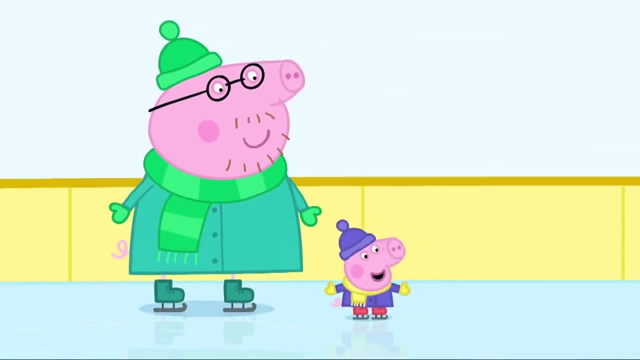 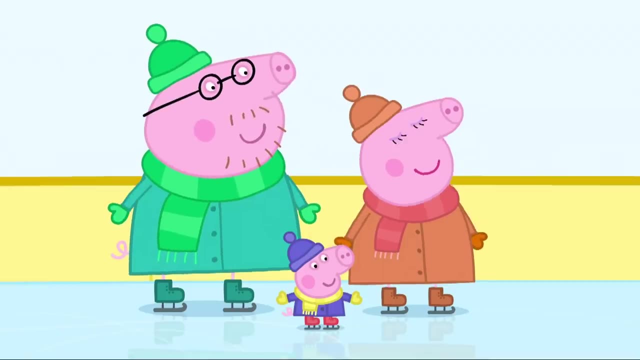 Well done, Peppa. Look at me, I'm skating. Peppa is doing really well. Yes, I'm a very good teacher. I'm going to teach Peppa how to skate. I'm going to teach Peppa how to skate. 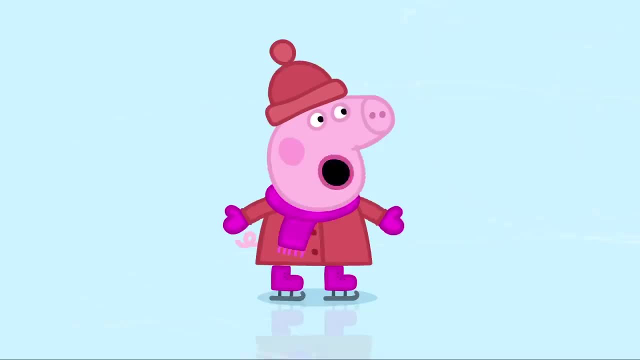 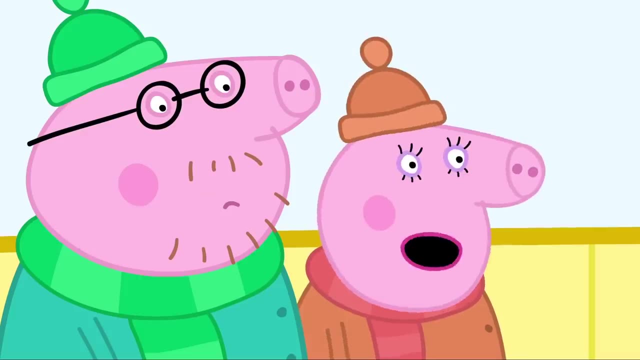 Slow down, Peppa, You'll bump into someone, Don't worry, Mummy, I'm very good at skating. Oh, where are the brakes? Oh dear, I forgot to teach Peppa how to stop, Oh. 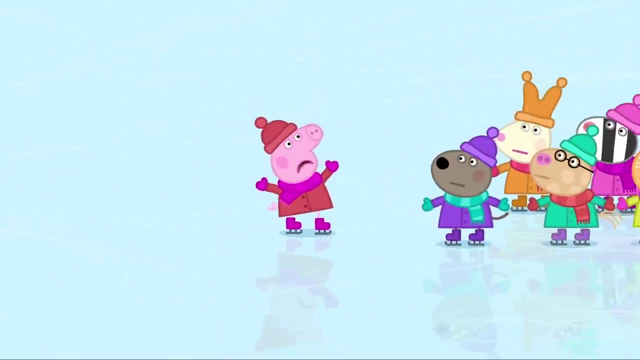 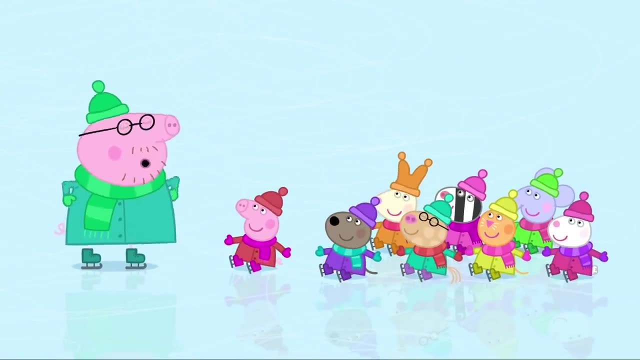 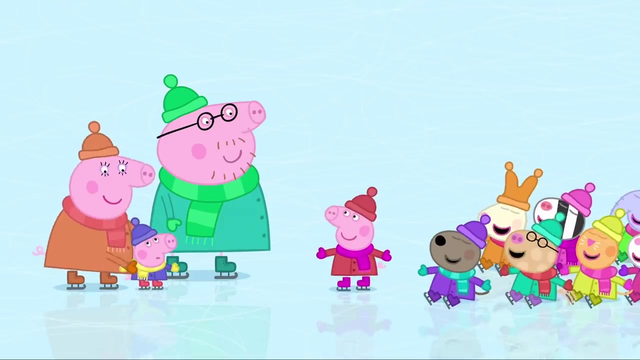 Ah, I can't stop. Look out. Whoa Ha-ha-ha-ha. Mummy Pig taught you how to skate, but I taught you how to fall over. Yes, I'm very good at falling over. George, do you want to skate too? 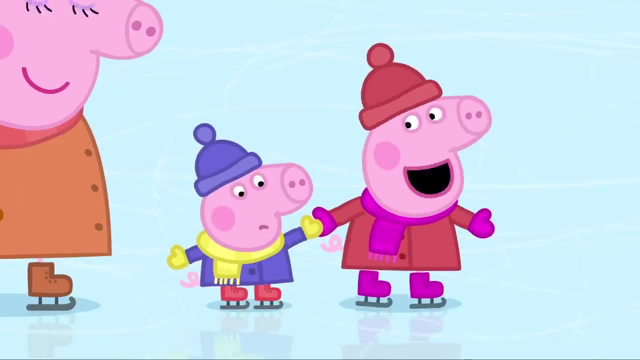 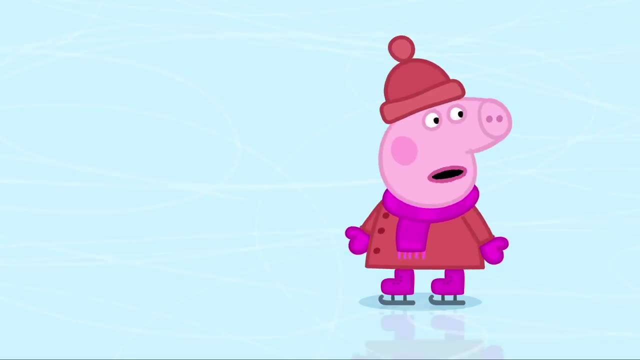 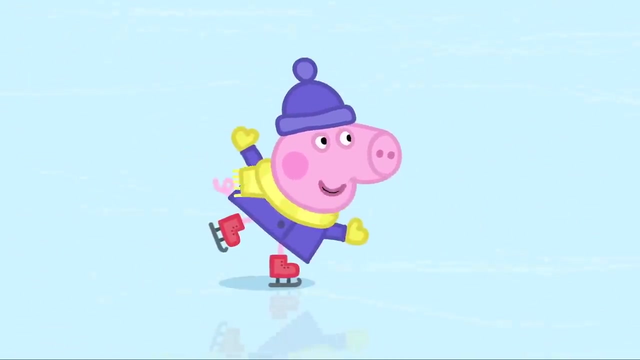 No, Come on, George, It's fun. I'll teach you. Hit him First. you need to Whee. George, come back, I'm teaching you how to ice skate. What a surprise: George can skate beautifully. 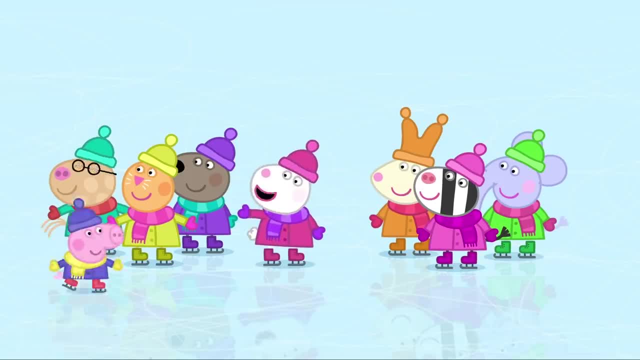 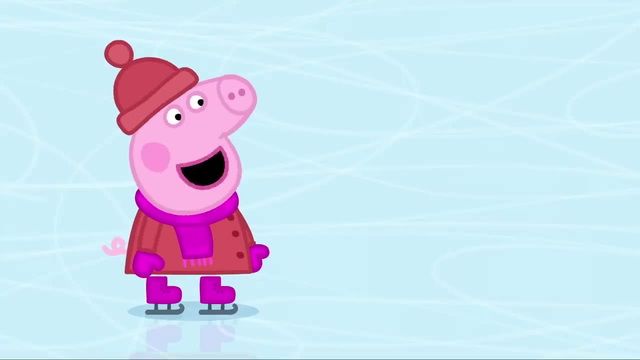 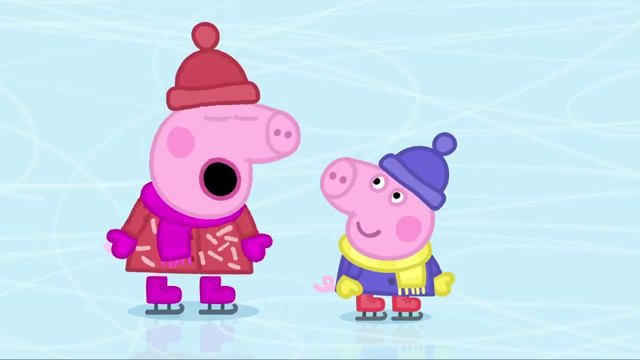 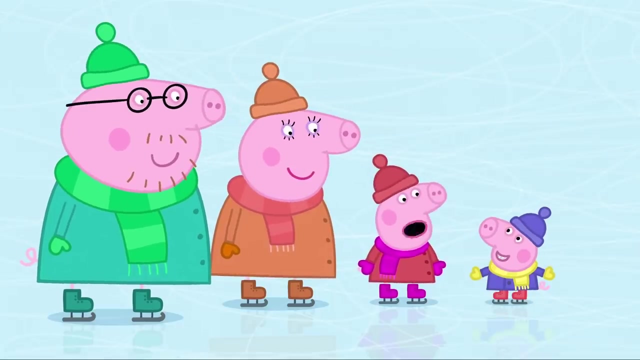 Wow, Look at George. Ooh, Very good, George. Now you need to learn how to stop Ha-ha-ha. Well done, George. You're fantastic, George. Yes, You did very well, George, for your first lesson. 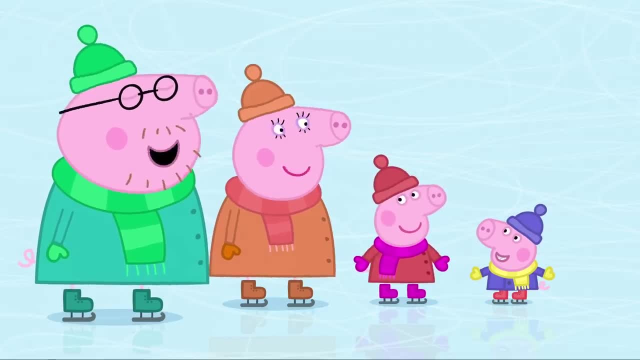 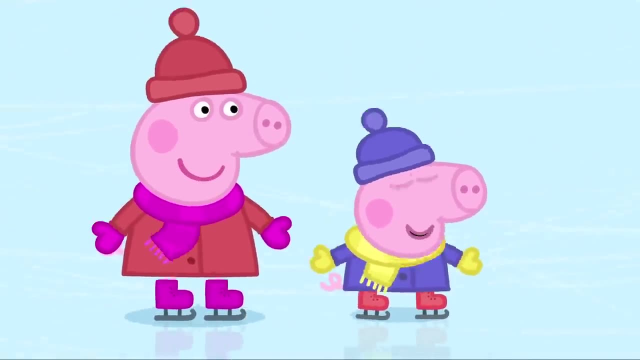 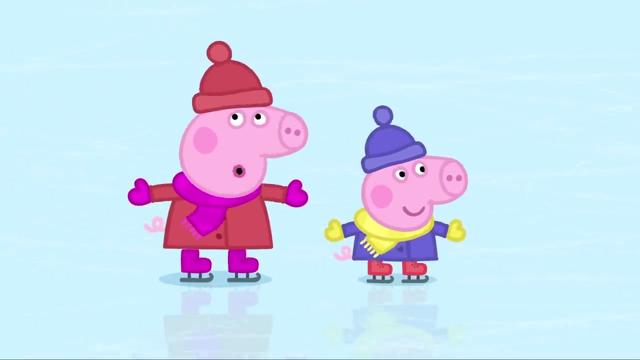 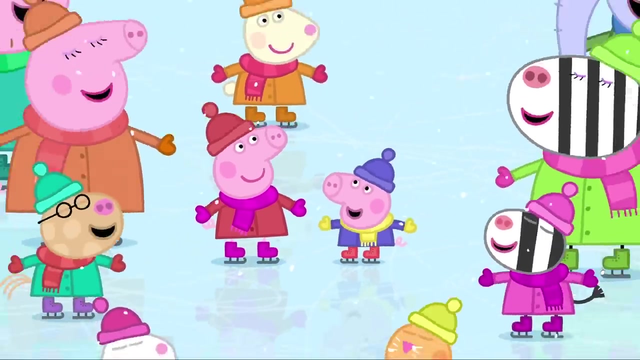 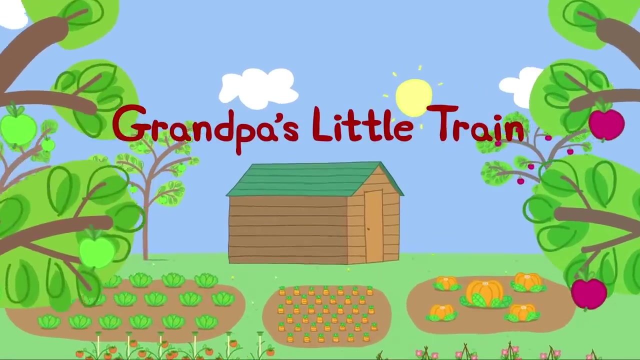 Yeah, First lesson. Come on, let's skate. Yeah, Peppa and George love ice skating. Everyone loves ice skating. Mummy and Daddy taught me how to skate, But I taught George. Peppa and George have come to play in Granny and Grandpa's garden. 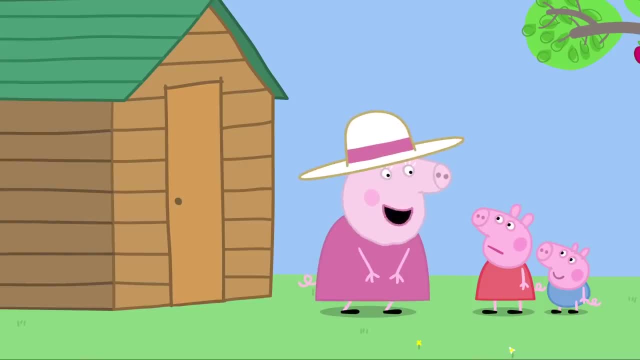 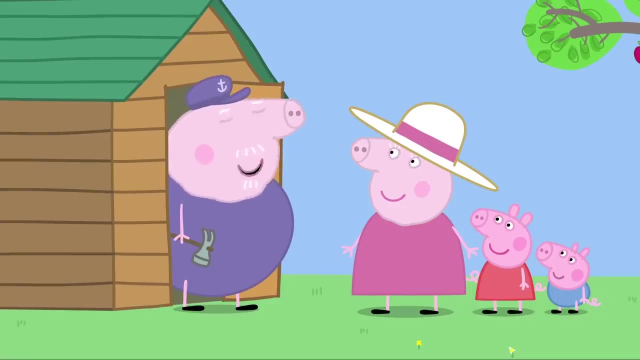 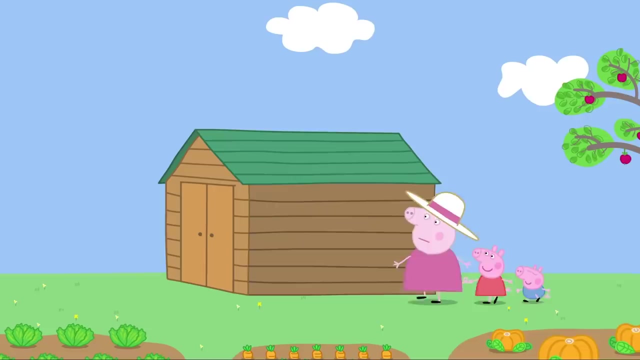 What's that noise? Grandpa's making something. Hello, Peppa and George, That's perfect timing. I've just finished making it And may we ask what it is? I'll show you. Wow, A little toy train. 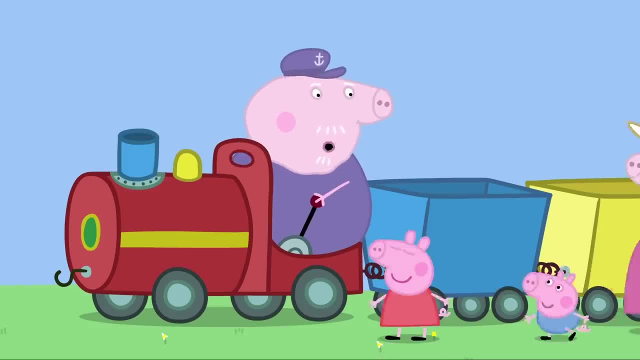 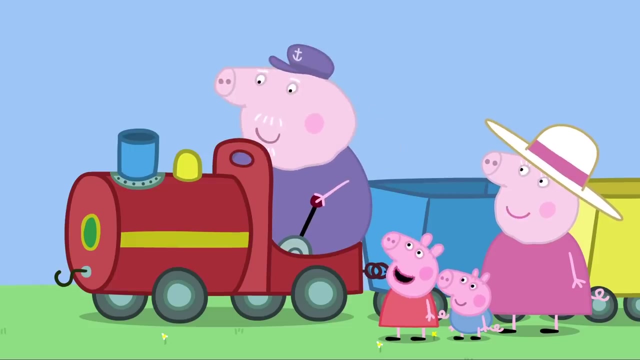 It's not a toy. This is Gertrude. She's a miniature locomotive, But doesn't it need railway tracks to run on? Oh no, I fitted Gertrude with car wheels so she can go anywhere she likes. Grandpa, can we ride in Gertrude? 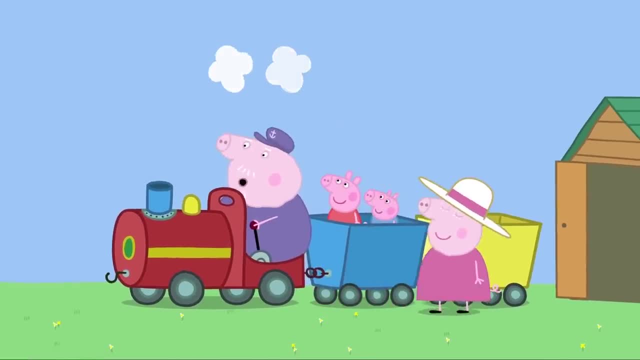 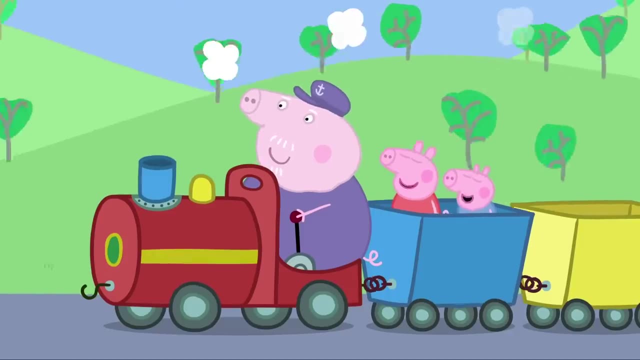 Hop aboard, Full steam ahead. Bye-bye, Granny, See you later. Peppa and George love Grandpa's little train. Grandpa's little train goes choo-choo-choo, Choo-choo-choo, choo-choo-choo. 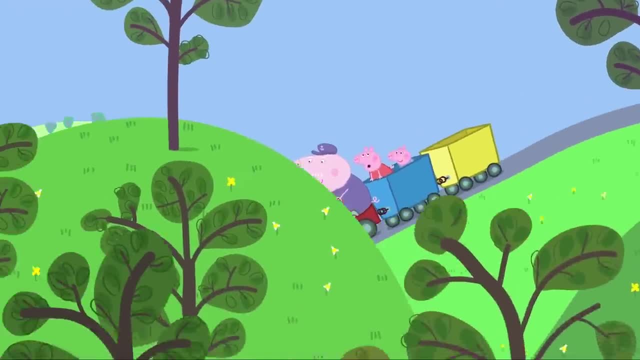 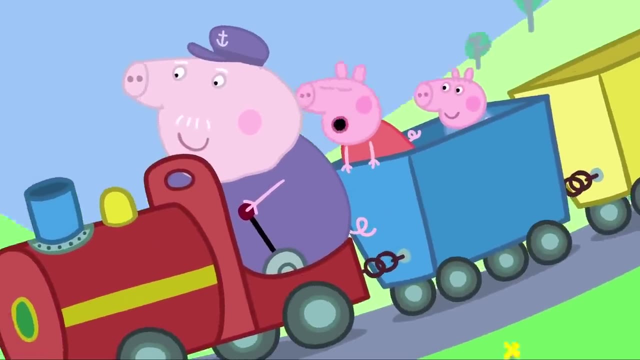 Grandpa's little train goes choo-choo-choo All day long And the piggies on the train go oink-oink-oink, Oink-oink-oink, oink-oink-oink, And the piggies on the train go oink-oink-oink. 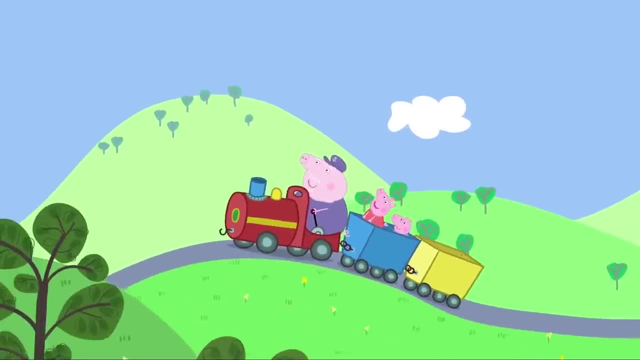 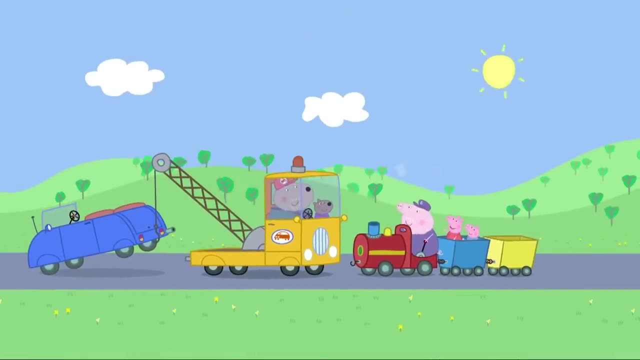 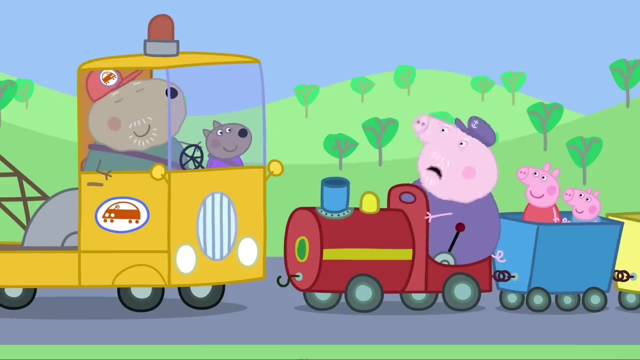 All day long. Here is Grandad Dog with Danny Dog. Hello, Hello Danny, I see you're playing toy trains. Toy Gertrude isn't a toy. How's your little lorry? Little lorry, My breakdown truck is a proper work vehicle. 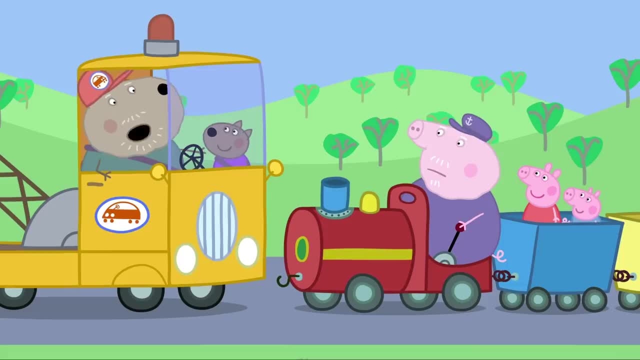 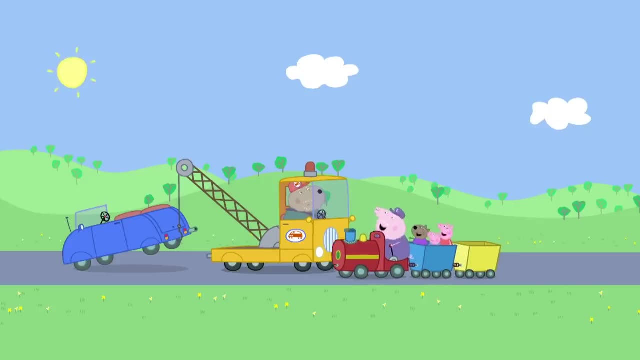 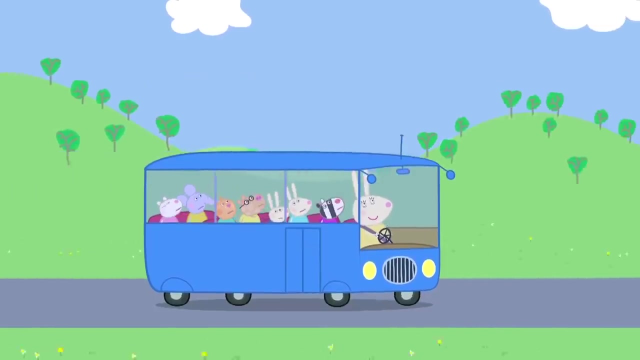 Grandad, can I ride on the train? It's your choice, Danny, If you'd rather play trains than. Thanks, Grandad, See you later. Miss Rabbit is driving the school bus, And to our left we can see some hills with trees. 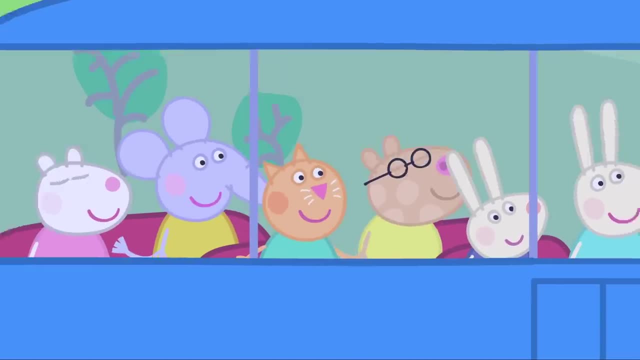 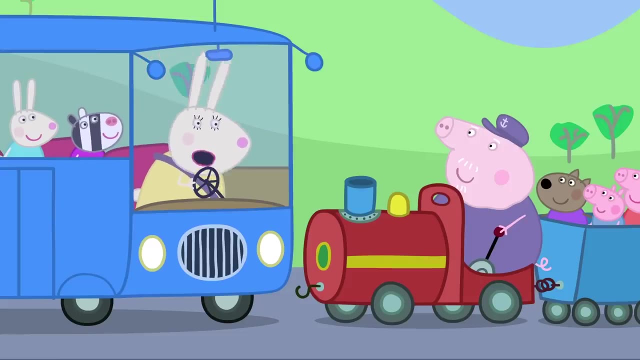 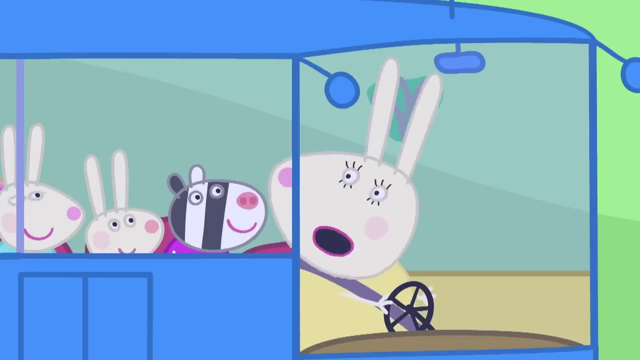 Hello everyone. Hello Peppa, All Peppa's friends are here. Can we ride on the train Um? I'm giving the children an educational bus tour. Are trains educational? They certainly are. Uh, hands up. 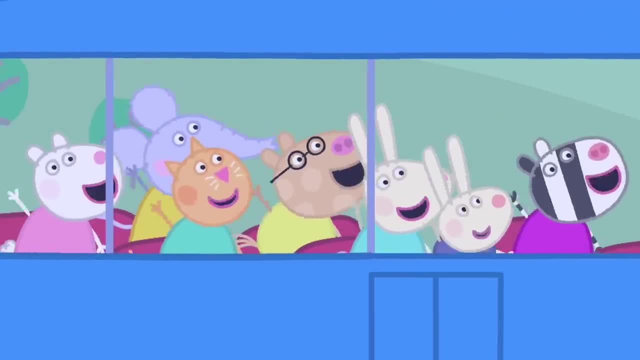 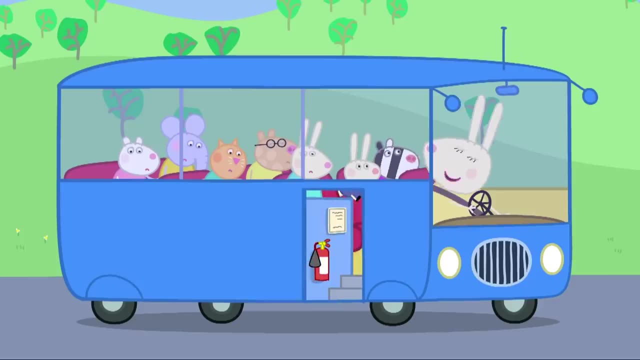 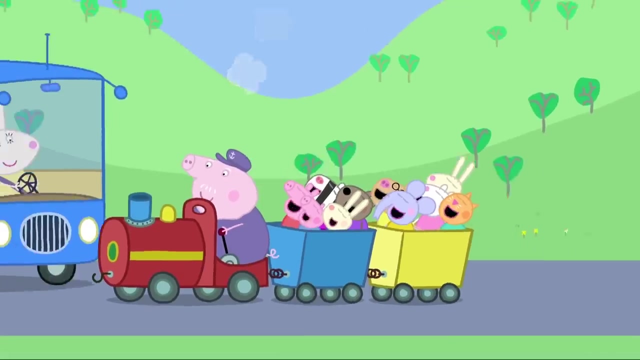 All those who want to ride on the train, Me, me And hands up. all those who want to stay on the bus. Okay, You can all go on the train and I'll follow along behind Meow, Grandad's little train goes choo-choo-choo. 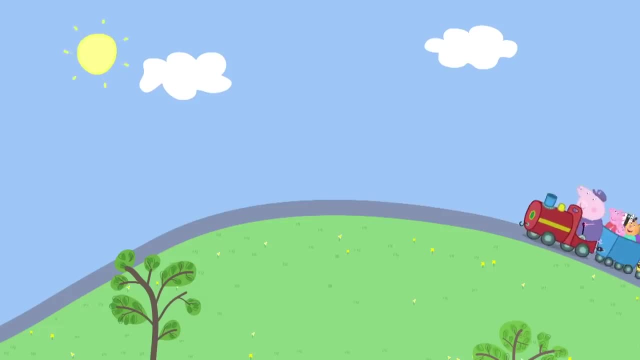 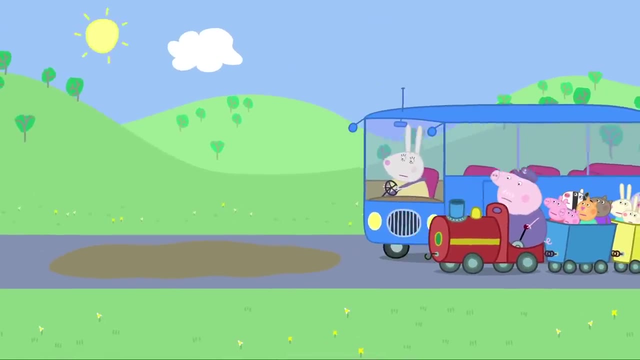 Choo-choo-choo, choo-choo-choo. Grandad's little train goes choo-choo-choo All day long. What a lot of mud. We don't want to get stuck. Maybe we should go a different way. 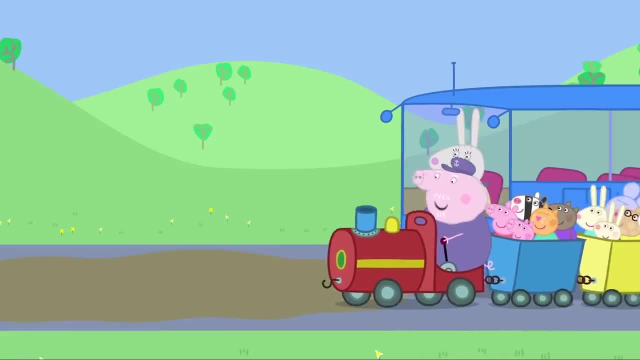 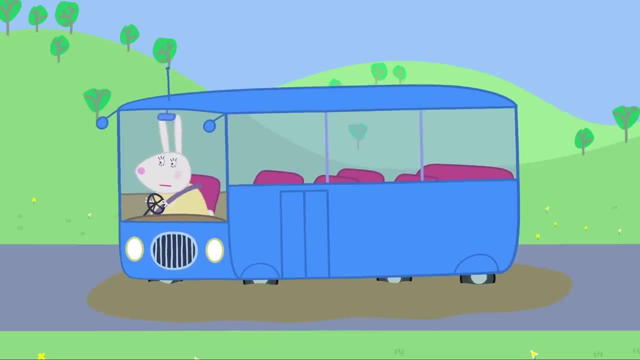 It's only a patch of mud. Come on, Gertrude, You can make it. Come on, bus, You can make it. Choo-choo-choo-choo, The bus is stuck in the mud. Oh bother. 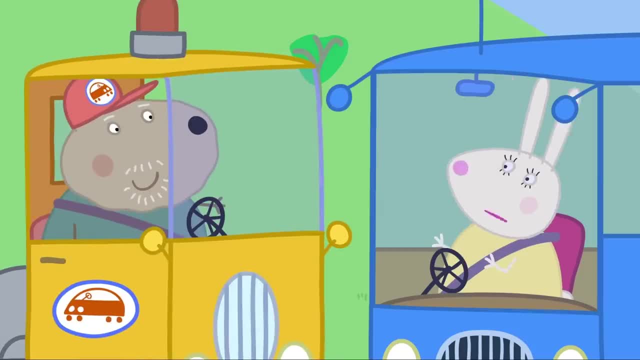 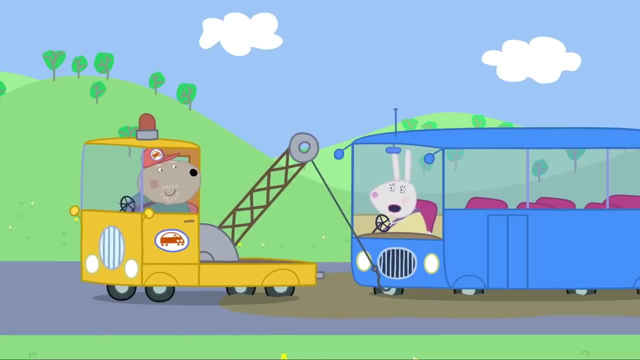 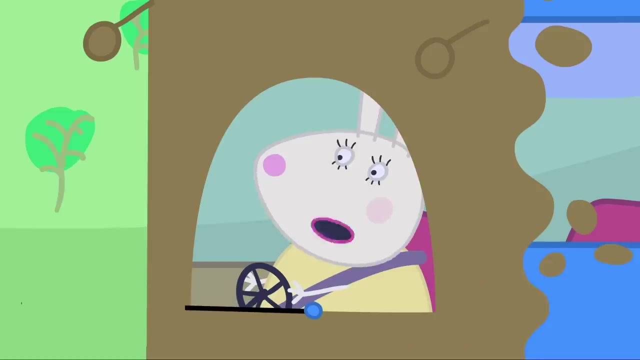 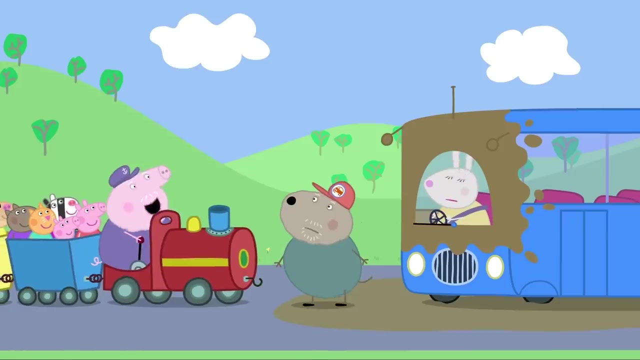 Hello Miss Rabbit. How are you today? I'm a bit stuck. Can you rescue me? Certainly, Is your truck strong enough. Trust me, Did it work? Er no, We need a vehicle with more power. Can I help in any way? 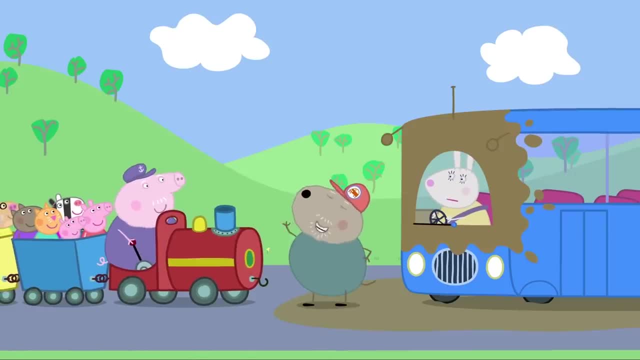 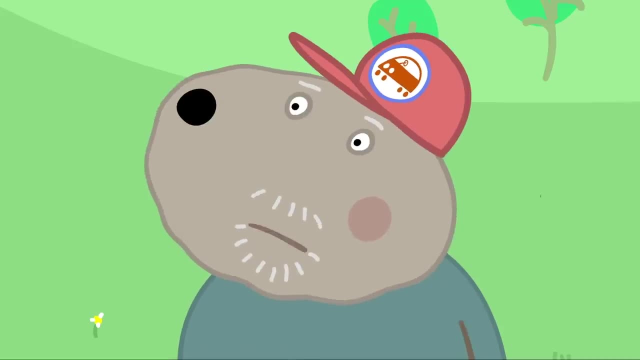 It's nothing that I can't deal with. Thanks. anyway, I've got an idea. Grandpa Pig's train can tow me out of the mud. Er good thinking, Miss Rabbit. Grandpa's little train is going to go choo-choo-choo-choo. 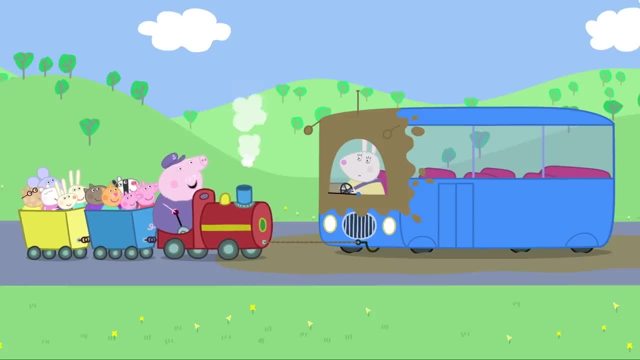 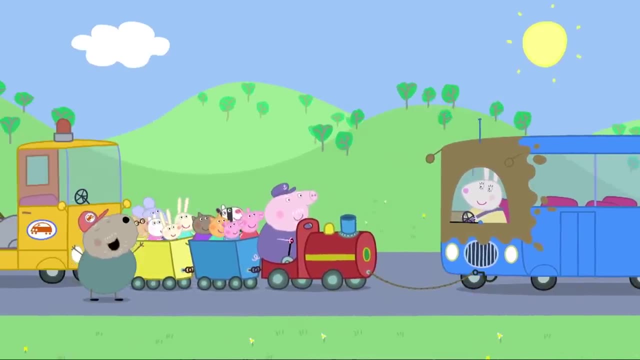 It's going to pull the bus out of the mud Full steam. Come on, Gertrude, Come on, Gertrude. Hooray, Ho-ho, well done. It's amazing what can be done by a toy train. 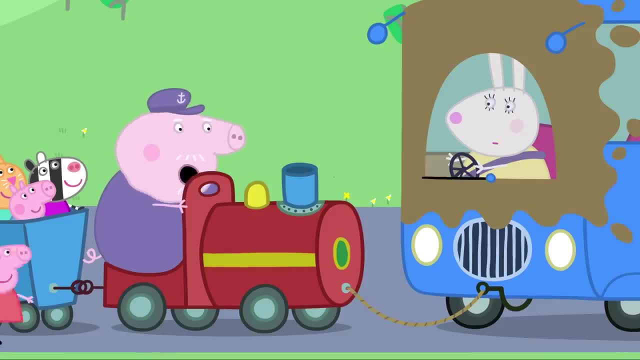 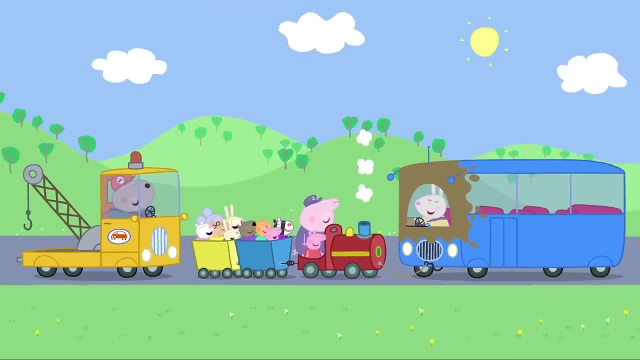 Toy Gertrude isn't a toy. Gertrude is the very best train in the whole world. Choo-choo-choo-choo-choo, Choo-choo-choo-choo-choo. 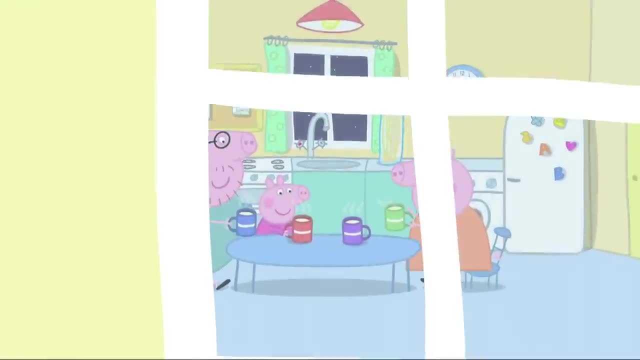 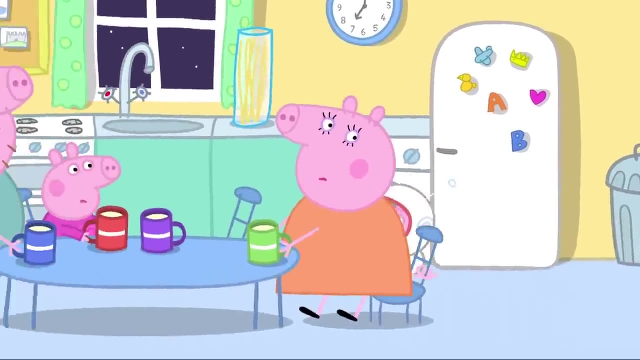 Stars. It is almost time for bed. Mummy Pig, Daddy Pig and Peppa are having mugs of hot milk. Choo-choo-choo-choo-choo. George, why are you dressed up in that spacesuit? 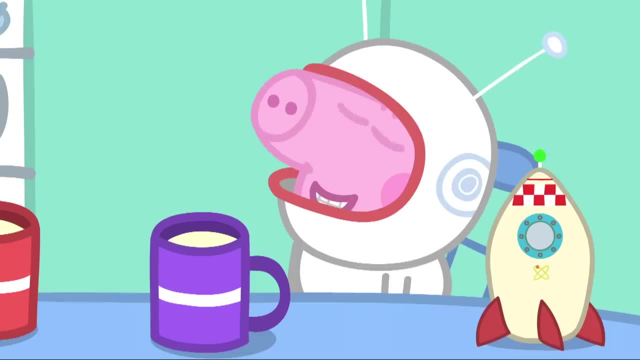 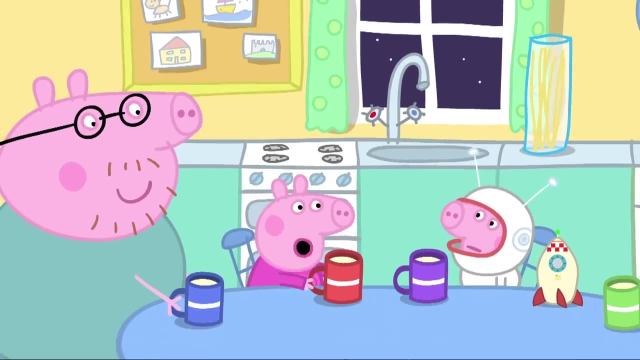 You should be in your pyjamas, Choo-choo-choo-choo. George loves everything to do with space, Choo-choo-choo-choo-choo. Oh, George, Get your space helmet off to drink your milk. 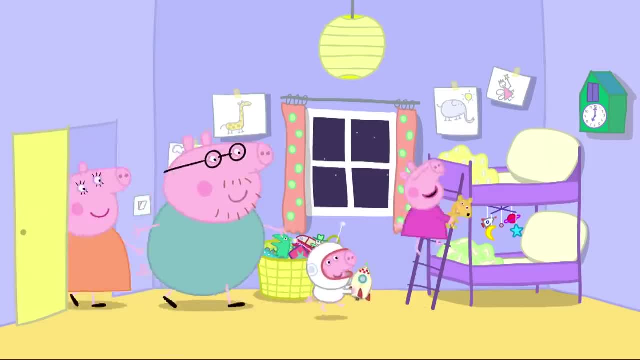 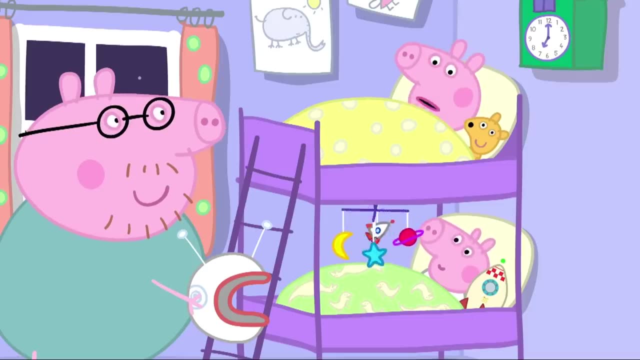 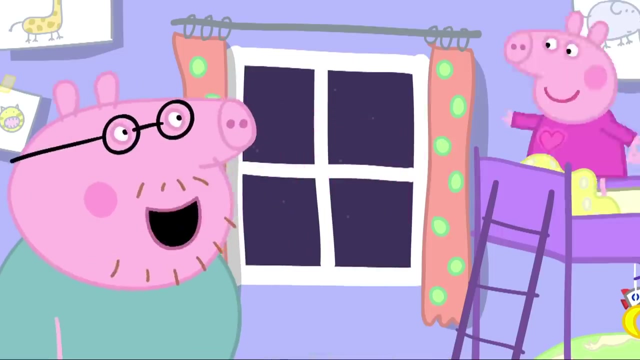 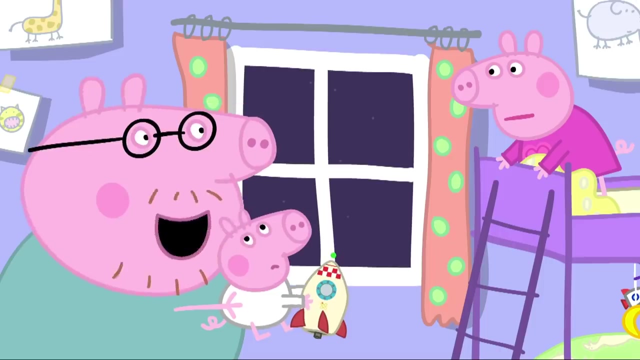 Bedtime little ones. At night, George likes to listen to his space mobile- Not space again. It's boring. Space isn't boring, It's full of stars. I can't see anything. It's too dark. It's easier to see the stars from outside. 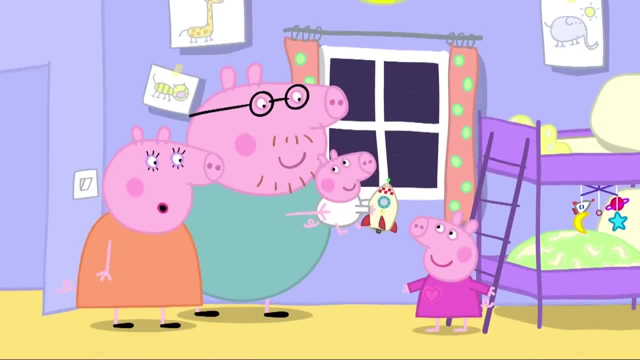 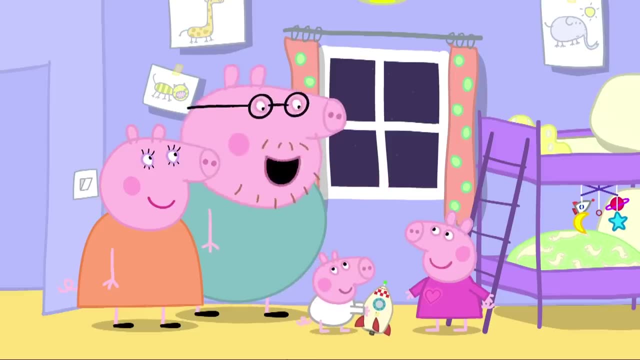 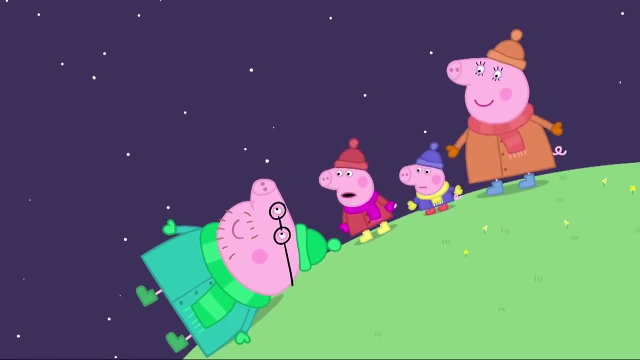 Can we go outside now? Peppa? you're in your pyjamas. Maybe if you put your coats on over your pyjamas, we could go outside just this once. Hooray Daddy, why are you lying on the ground? 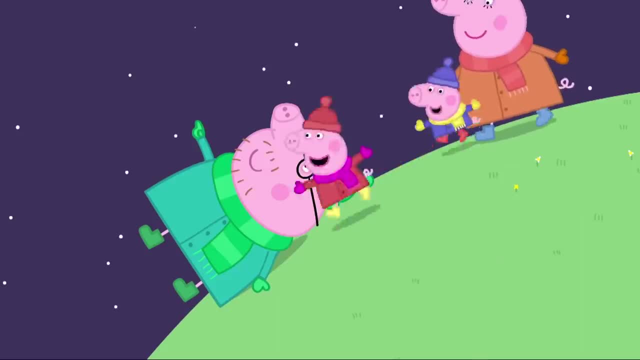 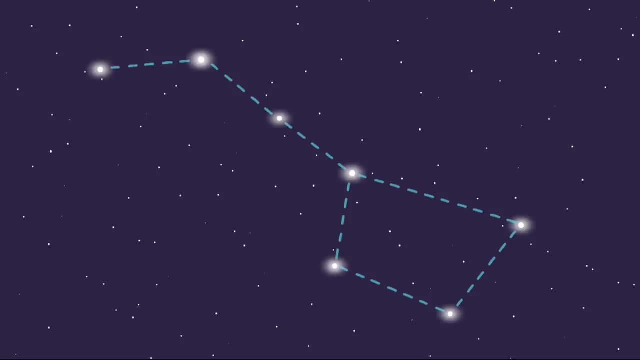 This is the best way to see the stars. Look at these stars. Imagine you are joining the dots. That's called the Big Dipper, Ooh, Yes. And the two stars at the end point to the North Star. Wow, North Star, North Star. 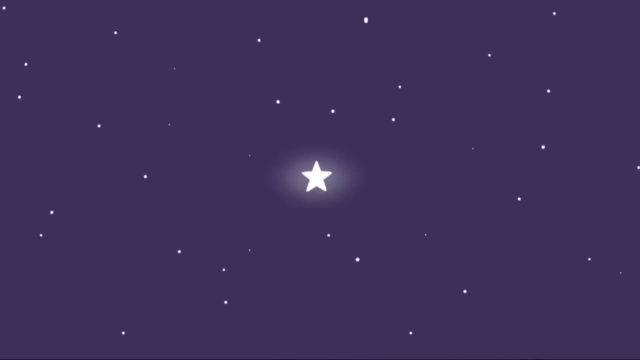 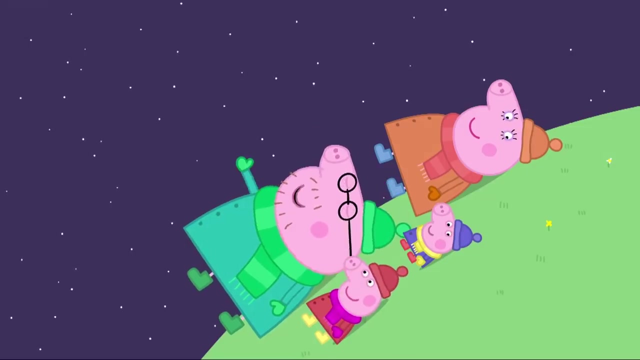 Are you near or are you far? Can we get there in the car? No, Peppa, The stars are much too far away. Are they even further than the seaside? Oh yes, they are. They are, Oh yes. 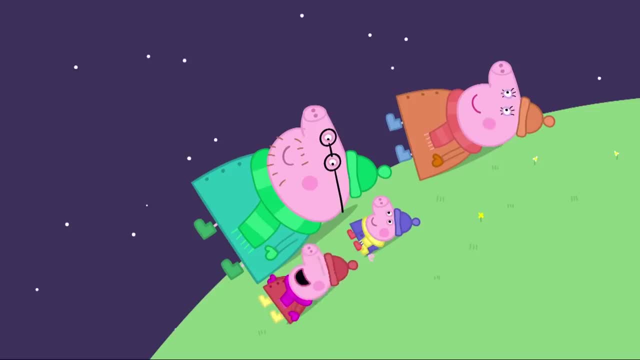 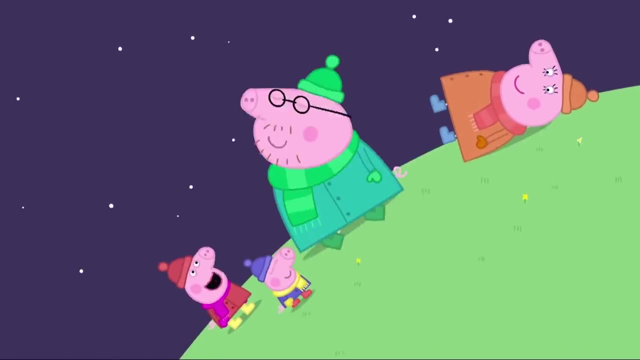 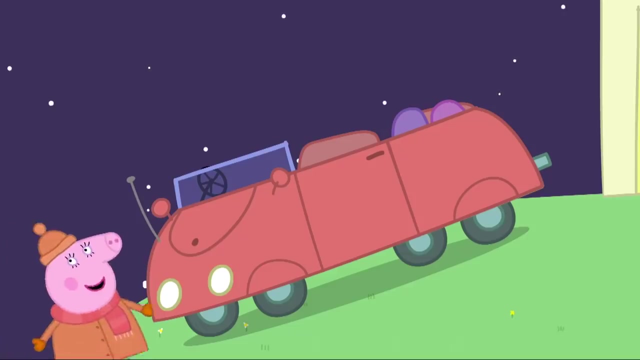 But they look a lot closer through a telescope. Have we got a telescope? No, but Grandpa Pig has a very good telescope. Can we go to Grandpa Pig's house now? It's much too late. Maybe we can go just this once, Daddy Pig. 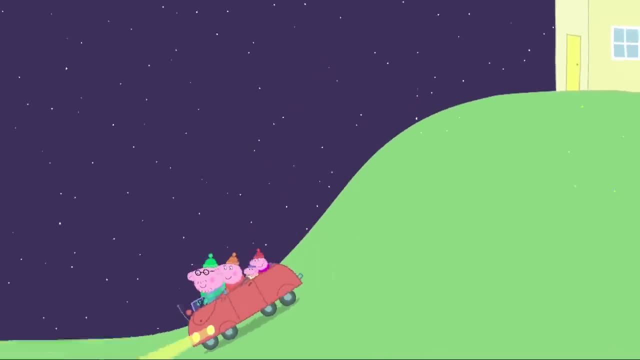 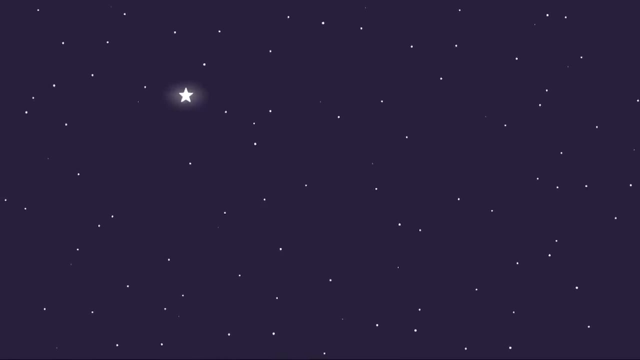 Hooray, It is the first time Peppa and George have been in the car at night. Look, We're following the North Star. HE GIGGLES. North Star, North Star, Shining with a twinkly glow. Please show us the way to God.